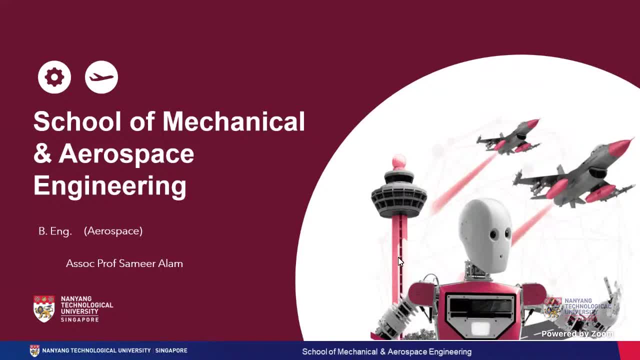 Hi everyone, a warm welcome to the School of Mechanical and Aerospace Engineering talk today. Today we have Prof Samia from the Aerospace Engineering to share with us a bit more about the degree program under the Aerospace Engineering. So in about two minutes time. 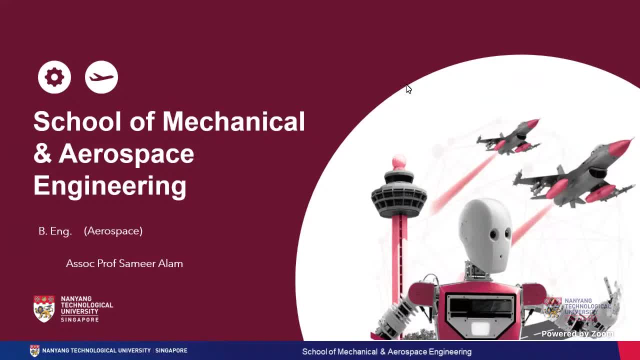 we will commence our sharing session. If you have any questions, feel free to drop them in the comment box or leave them on Slido. address them to Prof Samia and we will get to them during the Q&A session. In the meantime, make yourself comfortable and we'll be right. 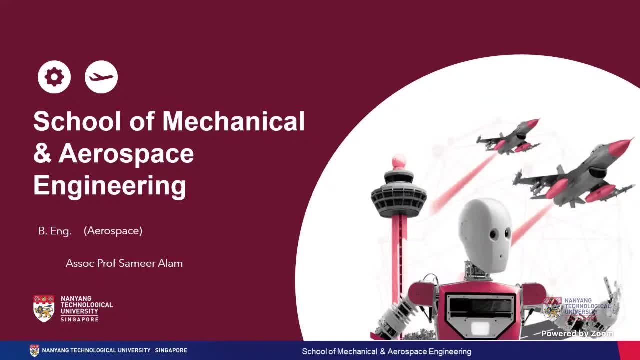 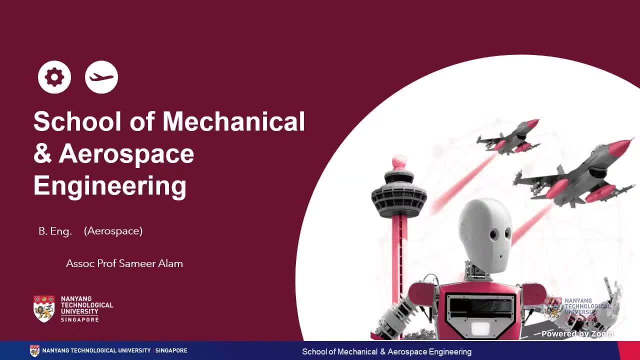 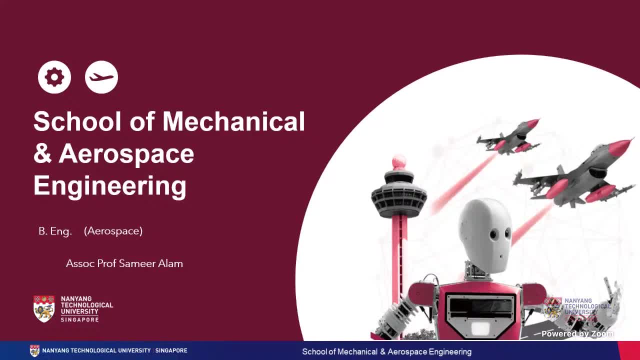 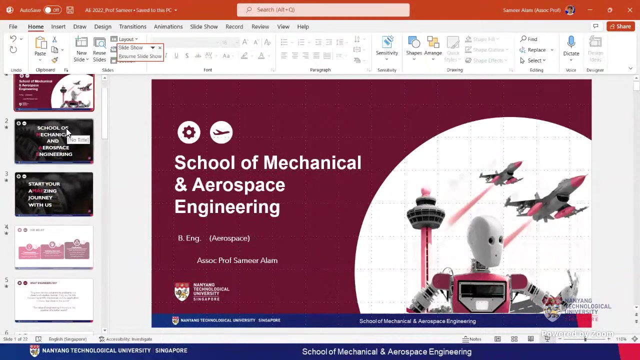 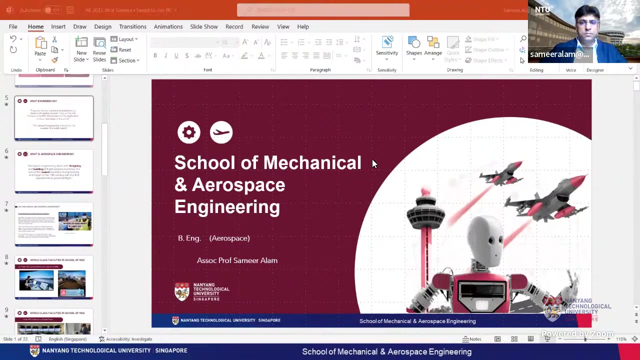 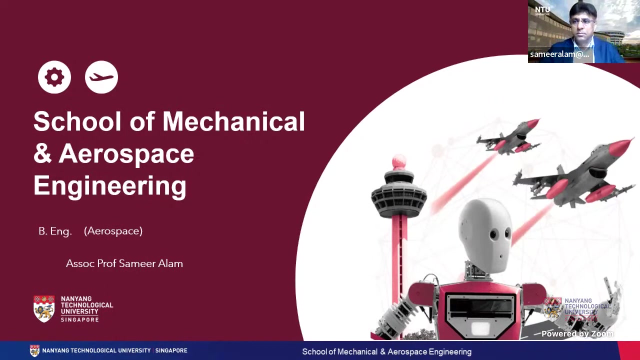 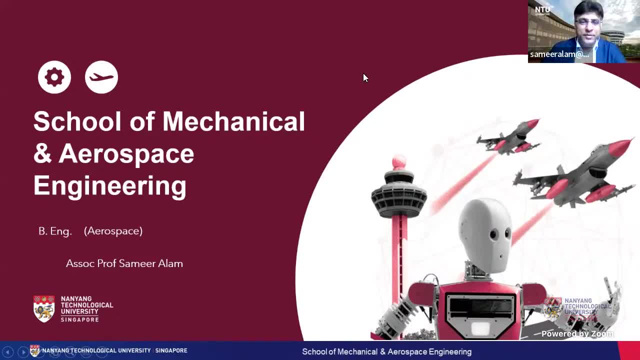 Thank you, Aline, and good afternoon. good noon everybody, wherever you are. A very warm welcome to the presentation on behalf of the School of Mechanical and Aerospace Engineering. My name is Samir and I'm an associate professor in the school. 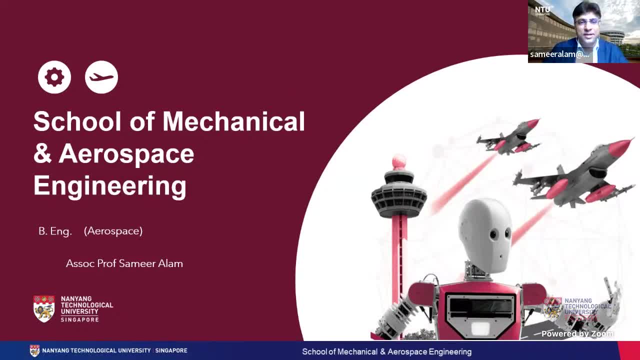 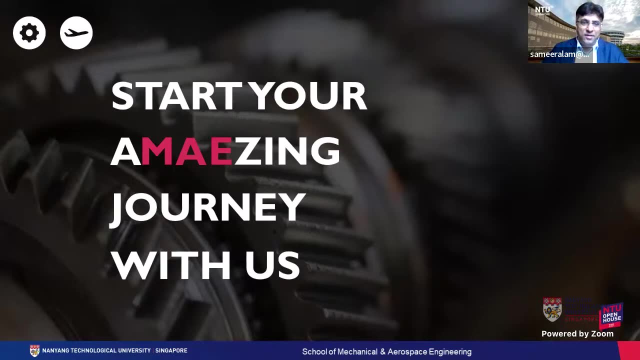 And I will be guiding you through some of the interesting things that we do in the school and hope that will excite you, motivate you to come and join the journey together. So we are the School of Mechanical and Aerospace Engineering And I want you to start your amazing journey with us to change the world, as engineers always do. 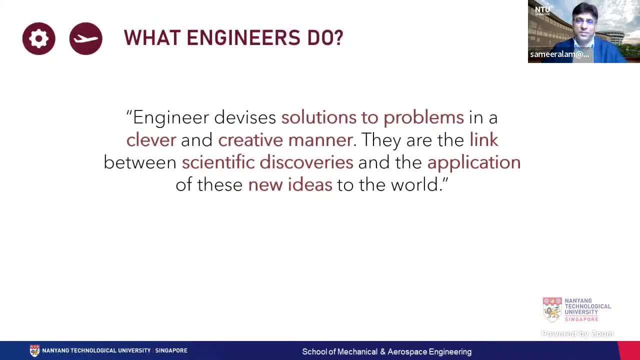 So you all know what engineers do, but let me give you a reflection: We don't just make things, We do these things in clear and creative manner. Actually, we are the link between all the scientific discovery and what you see in your hand: applications. 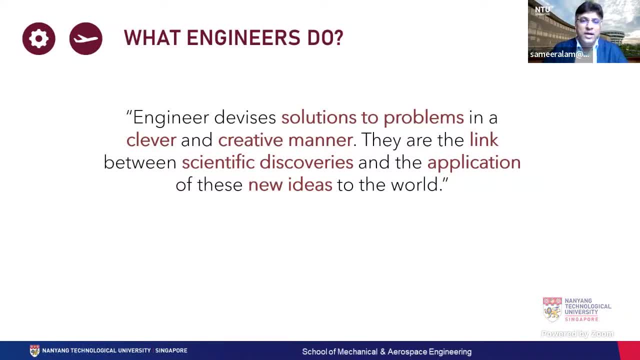 We are the connector, We are the translator. When these new ideas come to the mind of the scientist, we develop and deliver them to the society. This is what we engineers do. So this is what a value of engineer is: We create a better world. 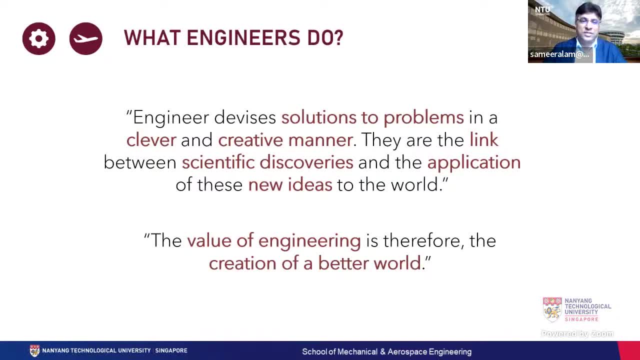 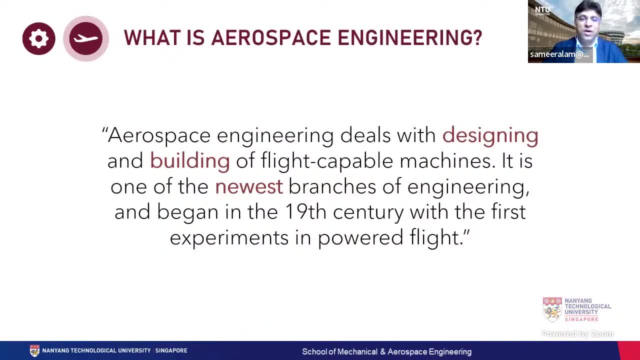 A better world which is safe to live in for every one of us. Aerospace engineering- the course broadly deals with the designing of flight capable machine And this is, as you know, one of the newest branch of engineering, started in 19th century with first experiments in the power flight. 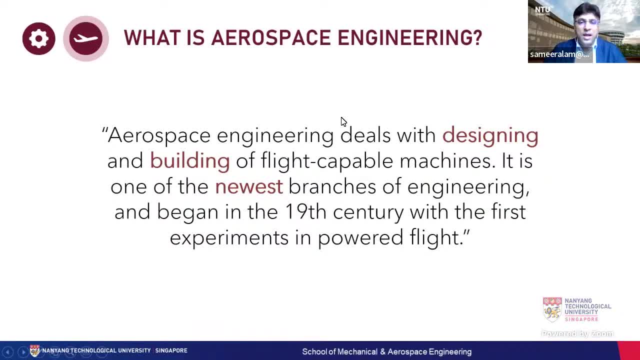 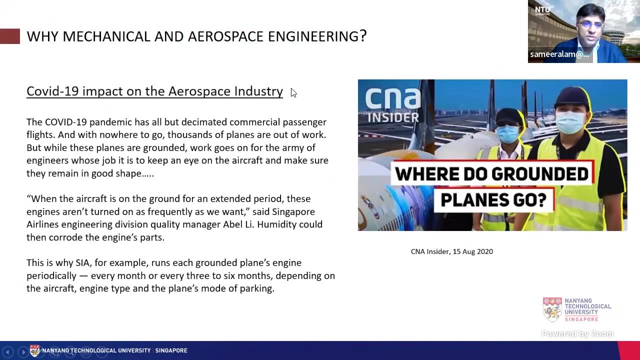 And that fundamentally changed the way people travel around the world. Today, aviation is an integral part- It is an integral part of how society moves around. during the COVID time, it had a significant impact on the society for the two years or very challenging, but aerospace engineers keep the ball rolling. 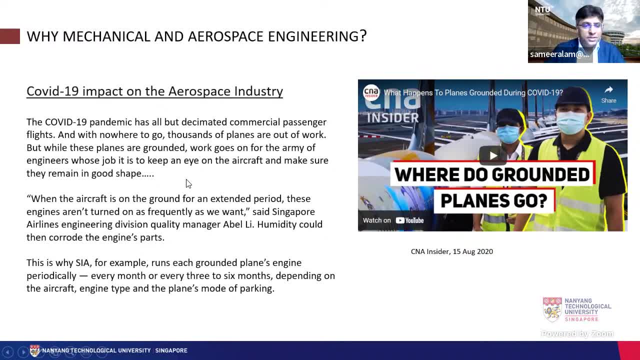 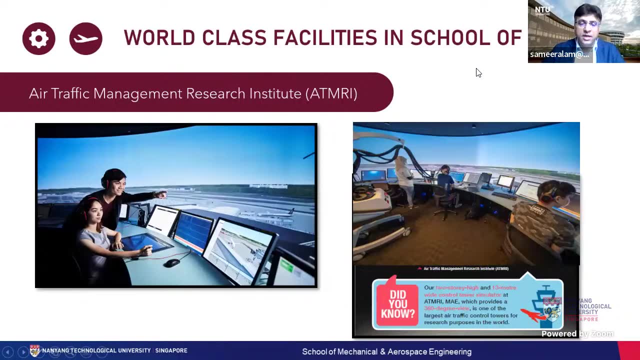 Let's watch by conducting regular checks, maintaining the engines so that everything is working efficiently. Let me quickly give you a Broad overview of the world class research facilities that we have in the School of Mechanical Aerospace Engineering, For example. we have an entire Asia Pacific. 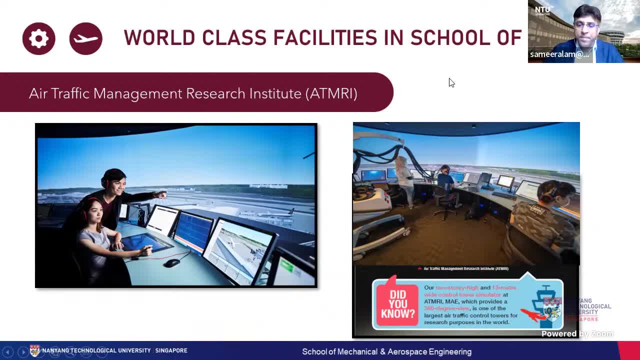 We are the only university to have a two story high, 30 meter wide air traffic control simulators at the Air Traffic Management Research Institute. This provides a 360 degree view for research and teaching purposes. for the students who are studying undergrads Make use of this facility for their lab experiments and research as well. 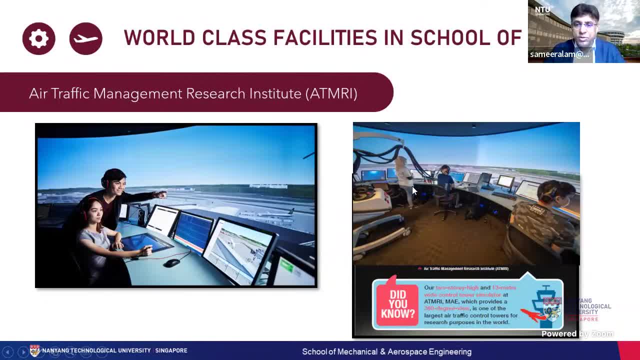 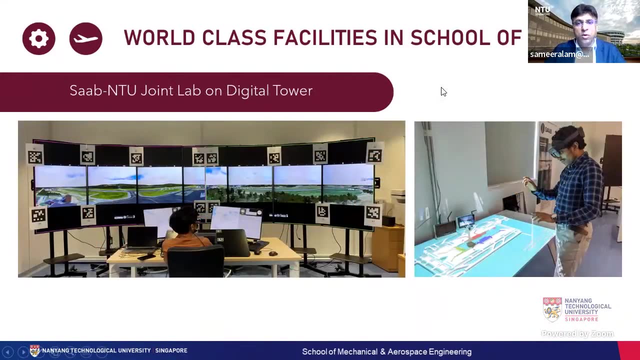 So, for example, on the right side you can see the MAE undergraduate students, FYPs, conducting experiments understanding the workload of the air traffic controllers while managing complex air traffic scenarios. Another lab that we have, which is also only three labs, are there in the world which have a digital tower laboratory. 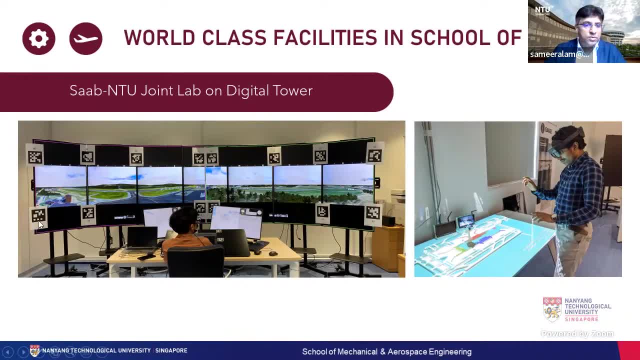 So on the right hand side you can see There is a digital tower laboratory which allows the air traffic controller to manage airport anywhere in the world without being physically present. Apart from the Cranfield University, Linkoping University, NTU is the only other university that has such advanced research facility for students to conduct research. 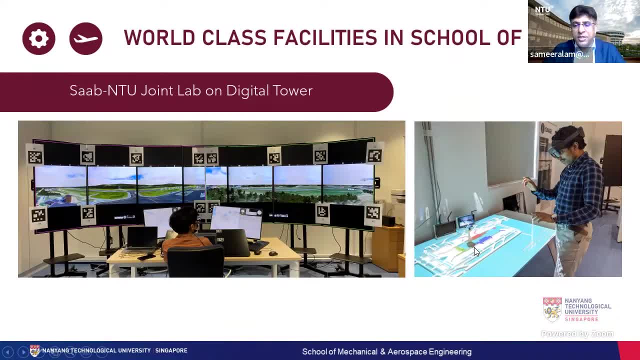 On the right hand side you can see there's a 3D printed Changi Airport Tower layout and the entire runway and taxiway. On the right hand side, you can see there's a 3D printed Changi Airport Tower layout and the entire runway and taxiway. 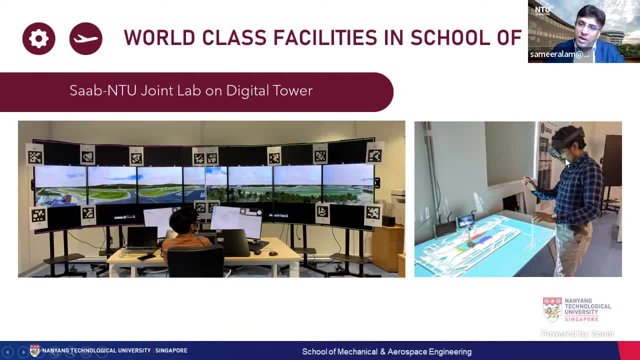 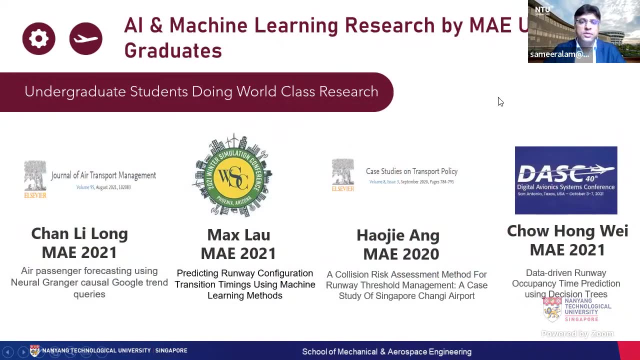 And this MAE student is using the HoloLens- a Microsoft HoloLens- to do a virtual reality interaction of managing the flight through human embodied gestures. MAE students are also doing world class research in artificial intelligence and machine learning to solve complex aviation problem. 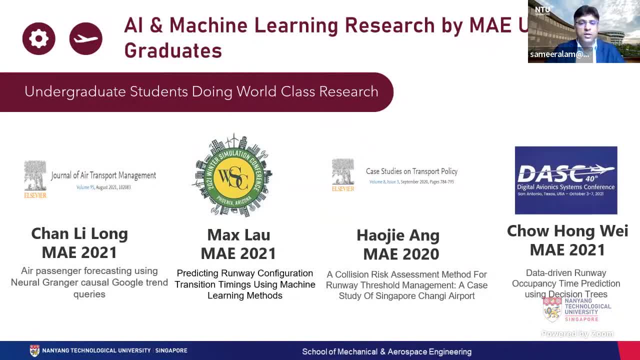 Our students have published research papers in top journals and conferences. Our students have published research papers in top journals and conferences Such as Journal of Air Transport Management, Winter Simulation Conferences, Case Studies on Transport Policy and Digital Avionics System and Conferences. 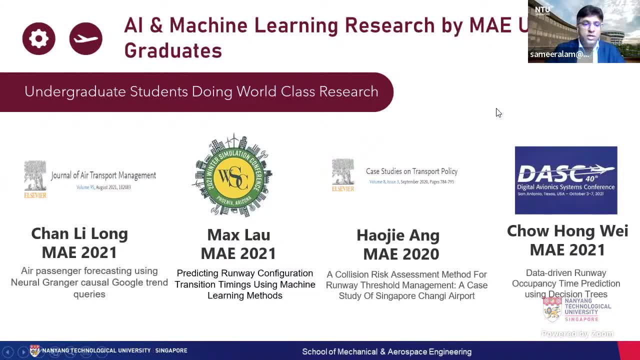 Such as Journal of Air Transport Management, Winter Simulation Conferences, Case Studies on Transport Policy and Digital Avionics System and Conferences. These students developed practical methods for air travel to be safe using machine learning and computational intelligence techniques. All undergraduate students. 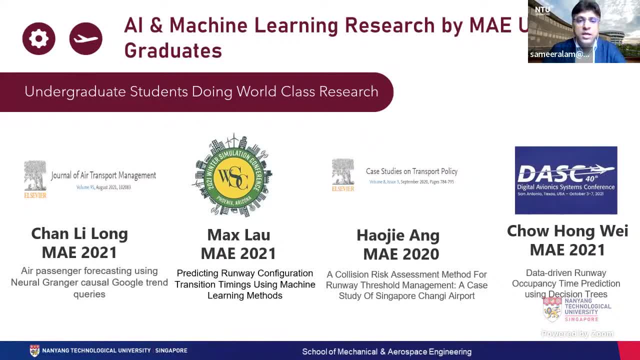 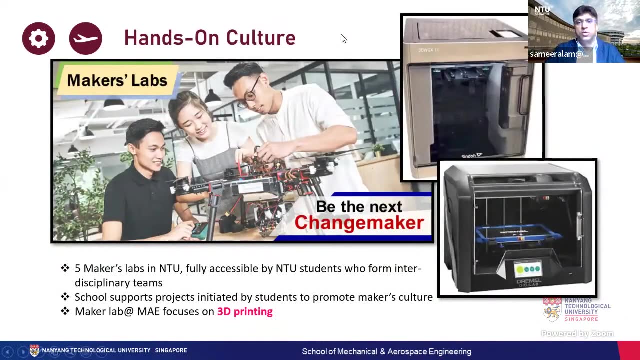 So students get an exposure, working closely with the professors To do Advanced Industry 4.0.. To do Advanced Industry 4.0. Focusing on AI and machine learning, solving the aviation problems. In the School of Mechanical Aerospace Engineering we have a hands-on culture. 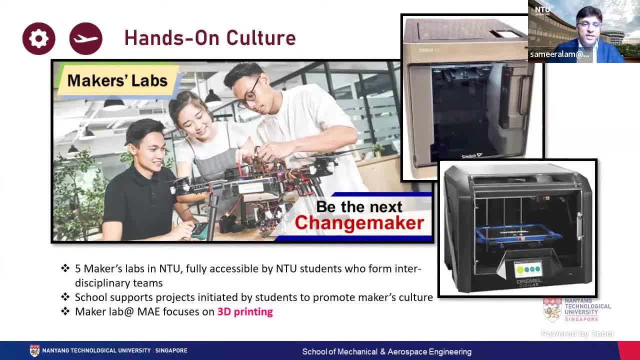 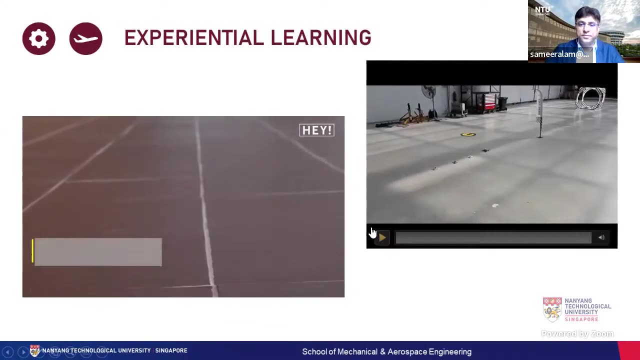 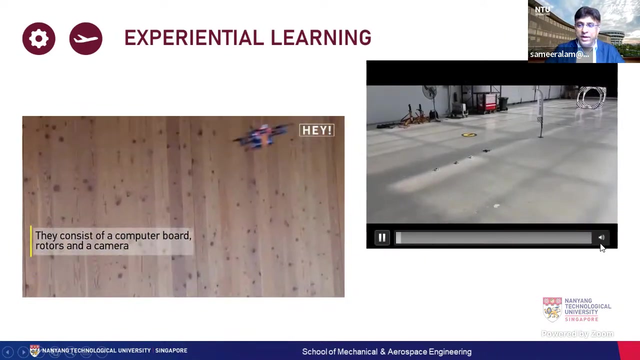 We have something which we call as Maker's Lab. This Maker's Lab allows NTU students to promote and develop their ideas and to do something hands-on. It involves very advanced 3D printing equipment where their ideas can take shape. Also, we have UAVs laboratories, which you can see over here in various videos. 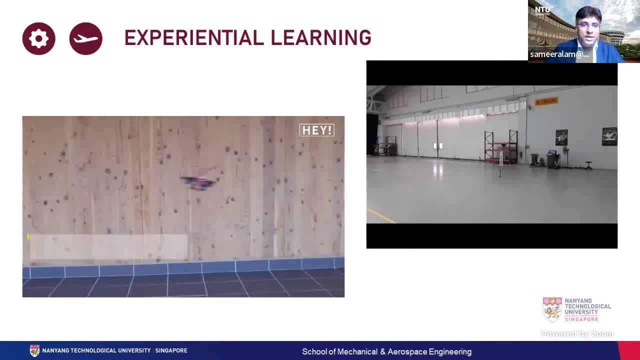 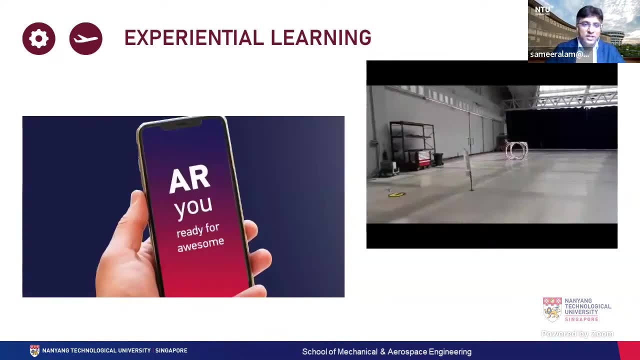 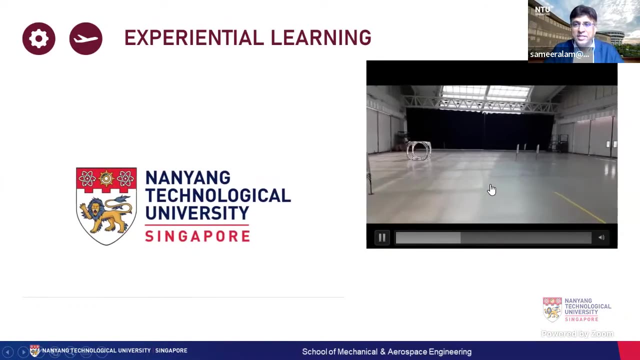 where students are able to play with new algorithms and models for drones to be detected, drones to be navigated and drones to race with each other. Also, we have systems and models that we have developed Where drones can play various games. Over here, for example, drones are doing air race using complex navigation obstacles and flying through it. 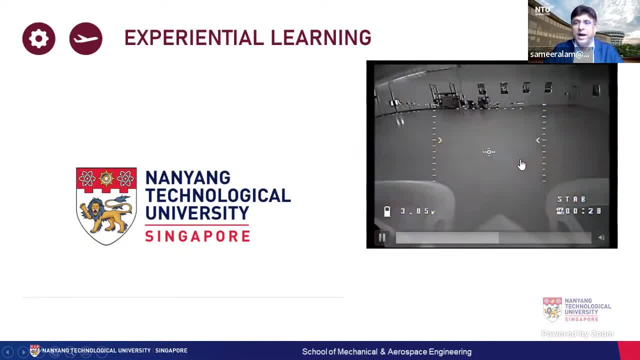 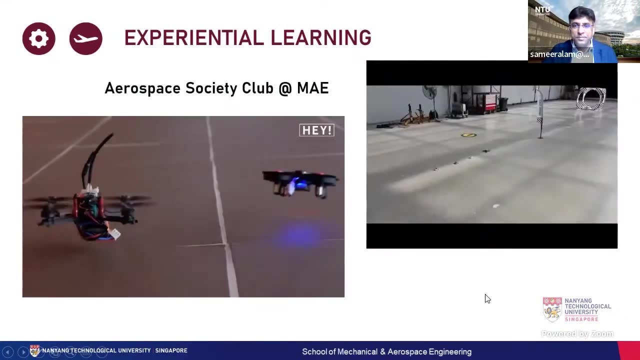 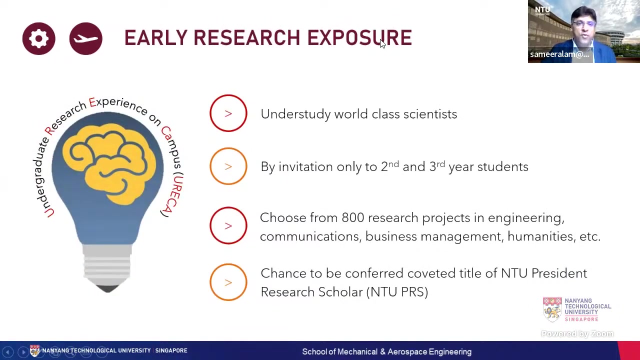 All of the algorithms and models are developed by MAE undergraduate students, So they are having a lot of fun in experimenting with new technology and developing state-of-the-art methods and models with the professors in MAE. MAE undergraduate students usually get very early research exposures. 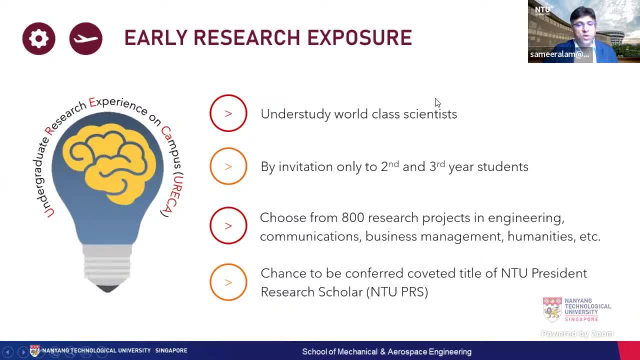 We do this through the Undergraduate Research Experience on Campus Program. This particular program is by invitation only to the second and third year students And they choose from around 800 research projects in engineering, communication, business management, as well as humanities. So this particular program strengthens 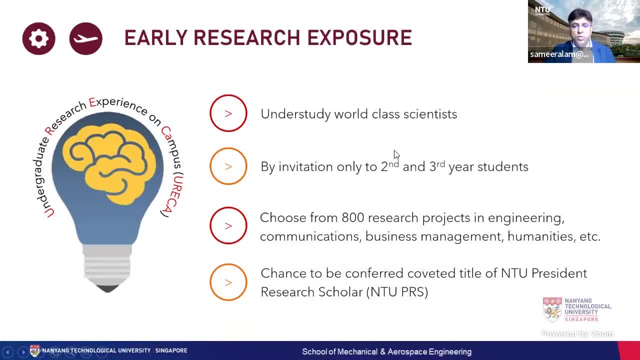 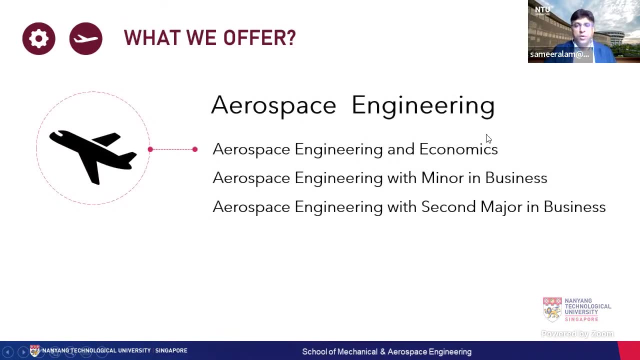 your cross-disciplinary experiences, You get the chance to be conferred a coveted title of NTU President Research Scholar as well. under the Eureka scheme, School of Mechanical and Airspace Engineering offer three combinations for the students to specialize. One is with economics, other with minor in business. 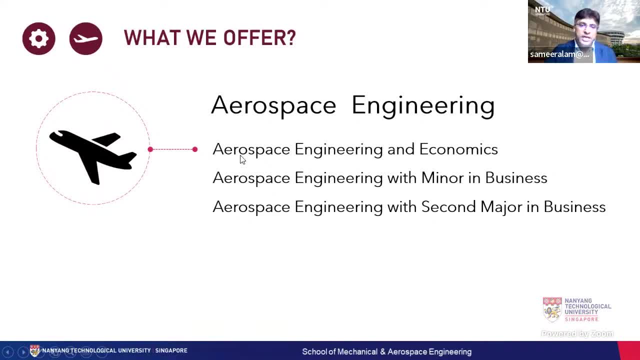 and the second is second major in business. This allows aerospace engineers to explore wider avenues in their life by exploring business opportunities and developing economic analysis and basically widening their horizon beyond going hard aerospace engineering, And they can do a lot of consultancy opportunities learning about that. 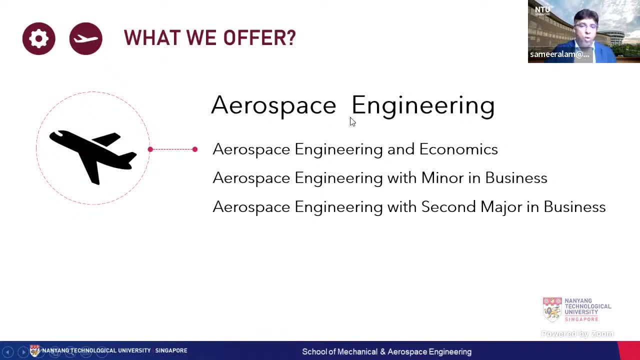 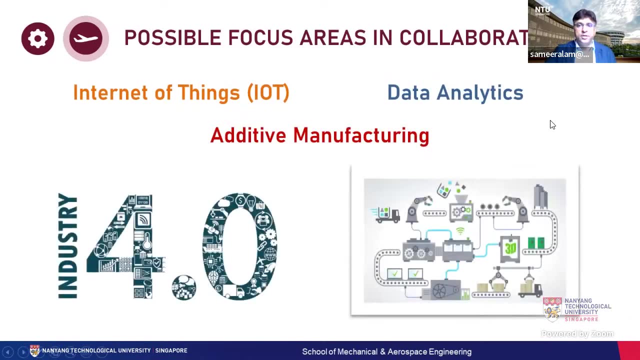 Many of our aerospace engineering students have gone ahead and opened a lot of startups And I think the knowledge that they gain in their major in business was very instrumental in that. There are various possible areas in the collaboration in the School of Mechanical Aerospace Engineering. 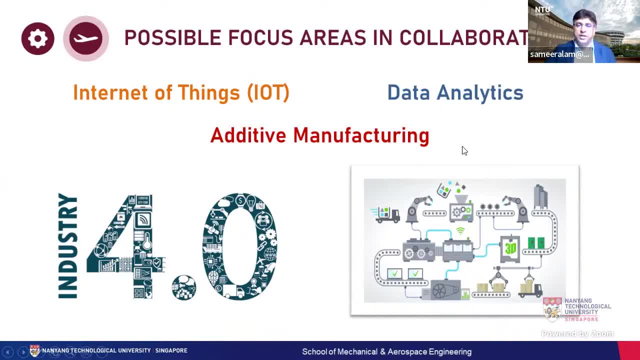 For example, Internet of Things, additive manufacturing, data analytics, and these all contributes to the next generation of industry, 4.0.. In the examples that I mentioned you before, MAE students are now at the forefront of the technology by using artificial intelligence and machine learning. 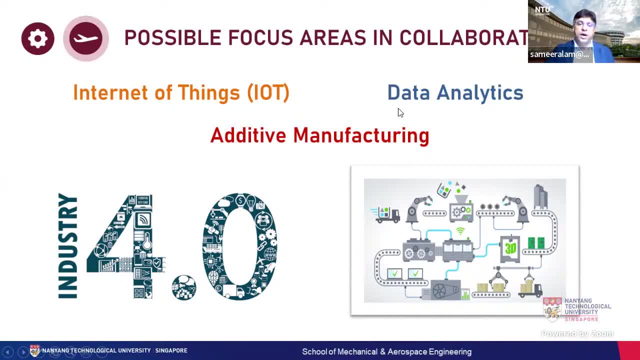 to solve complex aviation problem. We have a course for on AI and machine learning in the School of Mechanical Aerospace Engineering, where students are exposed early, first for the programming languages such as Python, and then on data sciences, as well as machine learning models and development. 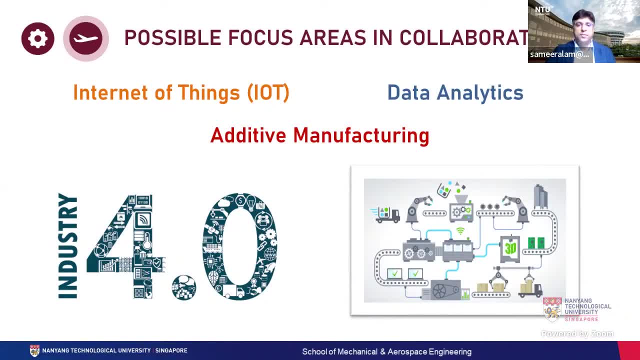 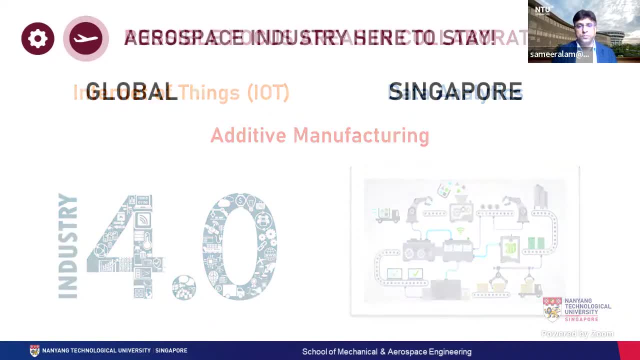 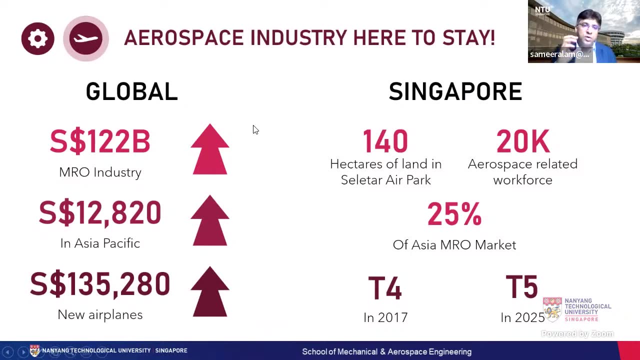 They carry on several projects during this course, making them expert level trained in using machine learning techniques for aviation-related problems. Aerospace industry in Singapore is here to stay. As you know, Singapore is a global aviation hub. We have over $122 billion MRO study. 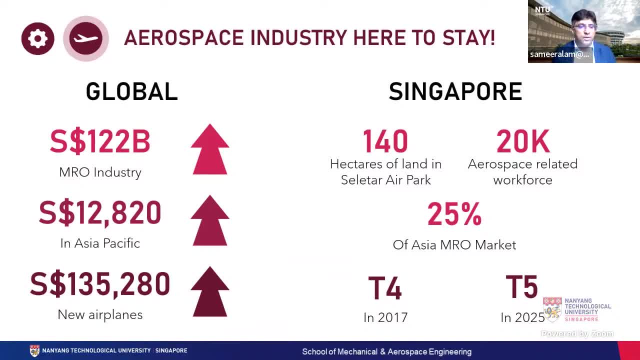 In Asia Pacific. we have over 12,820 industries in Asia Pacific. We have over $16 billion in industries over here. New airplanes we are procuring, as you have read in the news. Also, we have over 140 hectares of land. 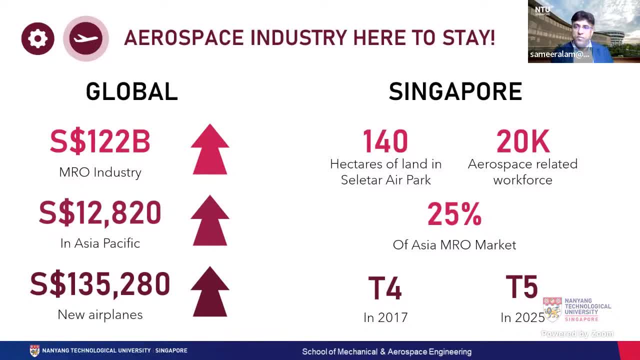 in the Salita Air Park that has been dedicated for aviation-related activities. We have aerospace-related workforce which is over 20,000, and 25% of the MRO market is here in Singapore. We are hoping to have T5 coming to life in 2025,. 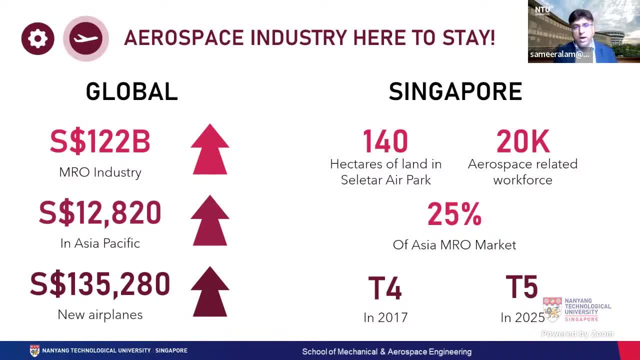 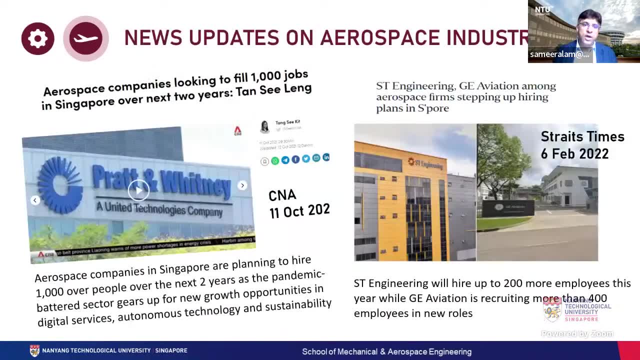 and then many engineers who have trained in aviation will be instrumental in that. Recently, you have seen many updates on aerospace industry for Singapore. Now aerospace companies are looking to fill thousands of jobs in next two years. Moreover, in-house companies and Singapore-based conglomerates such as ST Engineering, 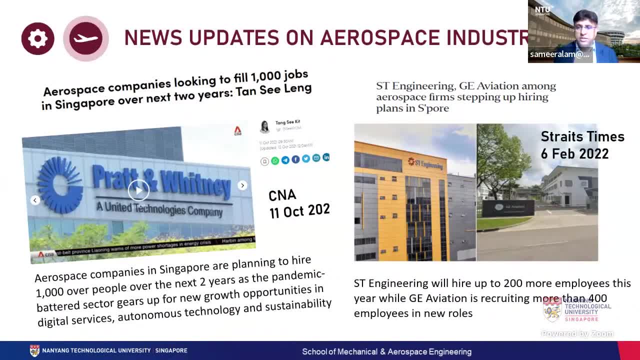 have upped their hiring plans. in Singapore, General Aviation is also recruiting more than 400 employees in the new role because there's so much demand for engine overhaul that's coming to Singapore, given the opening of the aviation sector. So next two years, three years, will be very exciting for aviation engineers. 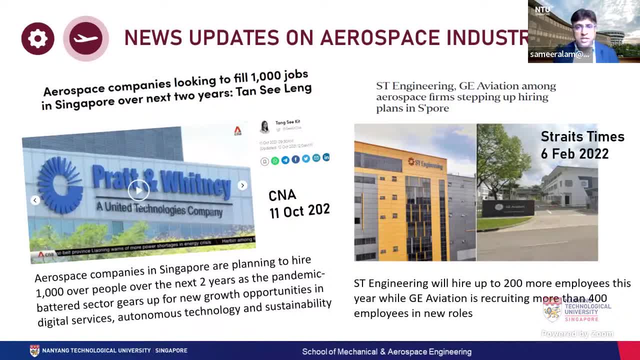 There will be a big uptake in the market that we will see for aviation-trained professionals Because of when the world is opening up. the travel is opening up. what connects the world? Aviation connects the world And who moves the aviation? You, the future aerospace engineers, who move the world. 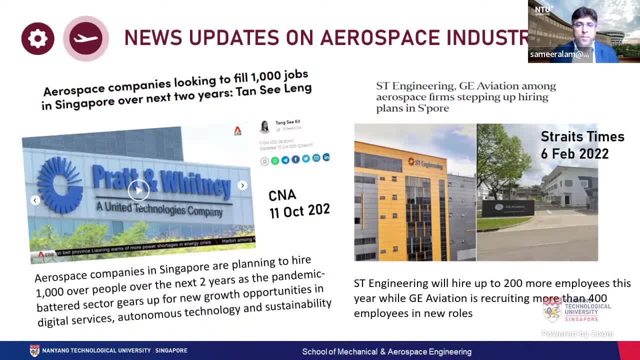 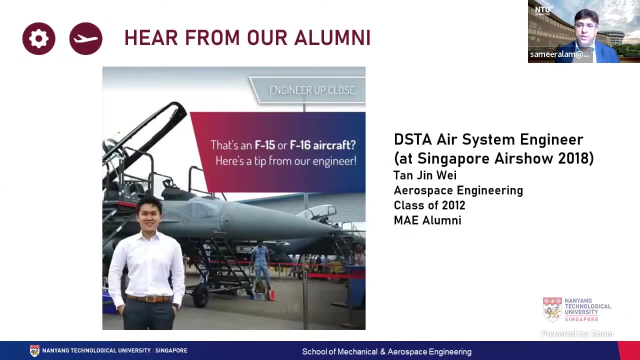 You will be required dearly in these multinational companies in Singapore and beyond. So don't lose this opportunity to be participating in transitioning the world Form a standstill Again to alive and kicking. Can you hear from our alumni? One is Jin Win. 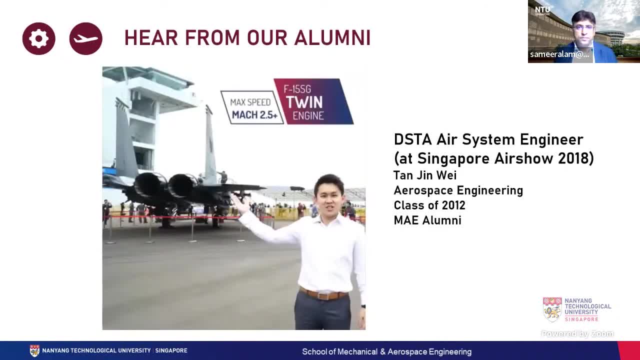 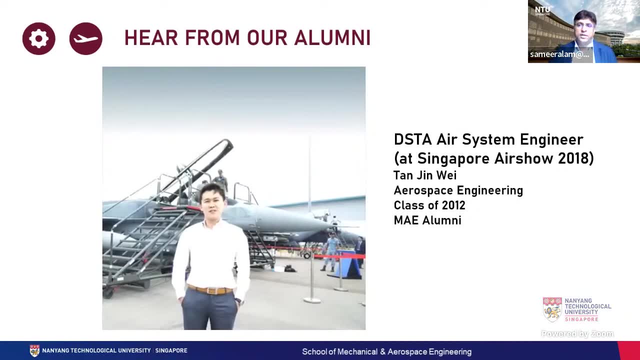 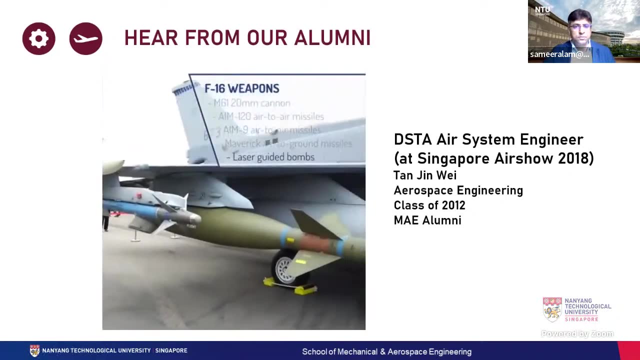 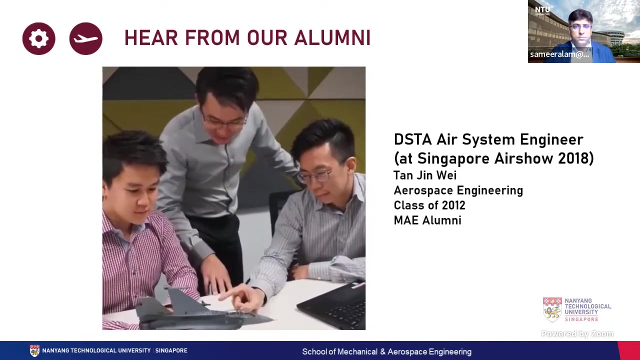 He is the DSTA Air System Engineer. He was involved in the design of F-16 Airspace Engineers. Correct, Yes, And the reason he was involved: This project should be done in Singapore, In Singapore, Yes, It is the first time I am doing this. 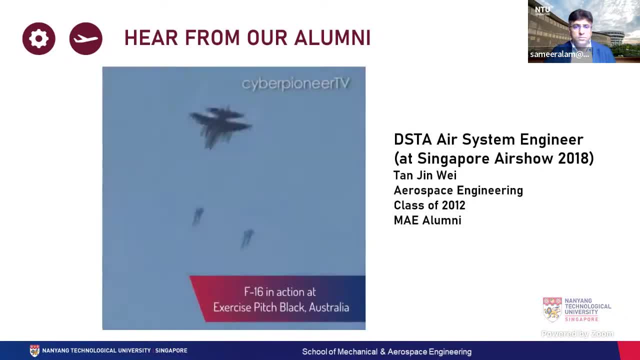 I'm very happy with the results. I'm very happy. Thank you, Joe, for putting this forward. Thank you, Eric, And now let me invite Dinesh Varan, our Master of Aviation Angular Engineering. Yes, please. Thank you very much. 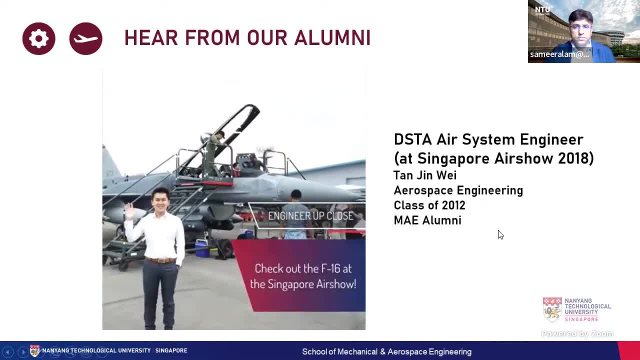 And even if you have not been trained, you might not be able to possibly continue in a company, And obviously things are going to change in a way that you wouldn't expect. So I encourage you to take a step back and be creative. 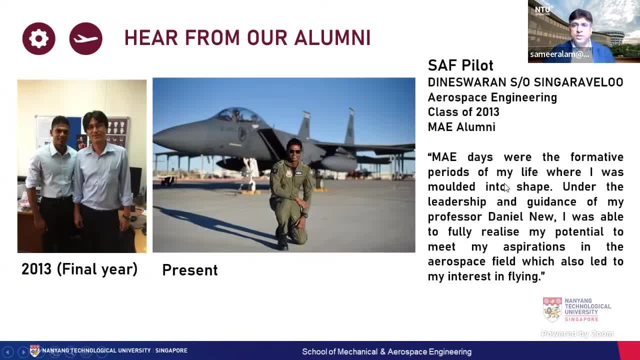 And hopefully you will find a way to create a better future And we do So. thanks you for coming, Thank you, Thank you, Thank you mentored him in the leadership and guidance and he was able to lead his aspirations and. 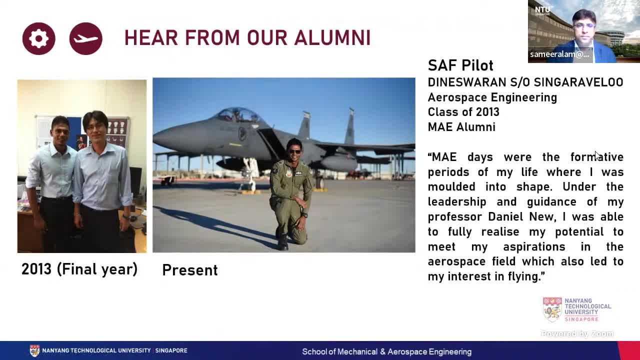 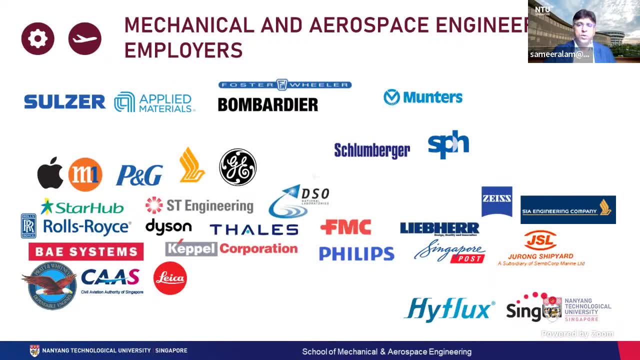 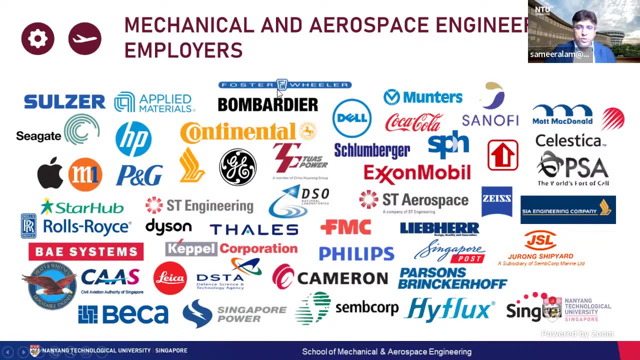 dreams to become SAF pilot. There are several aerospace and mechanical engineering employers in Singapore that are gearing up to participate in the opening up of the airspace air travel again, And I'm sure that you will be able to contribute to them when you start your journey with the. 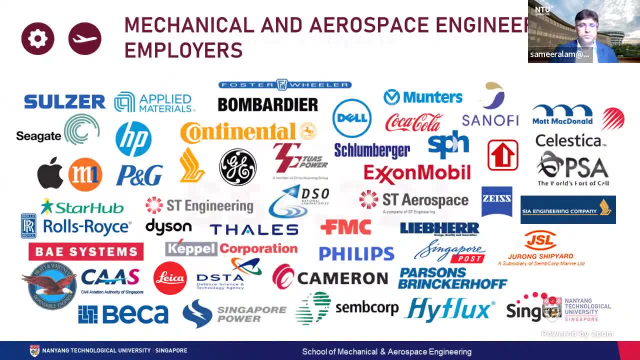 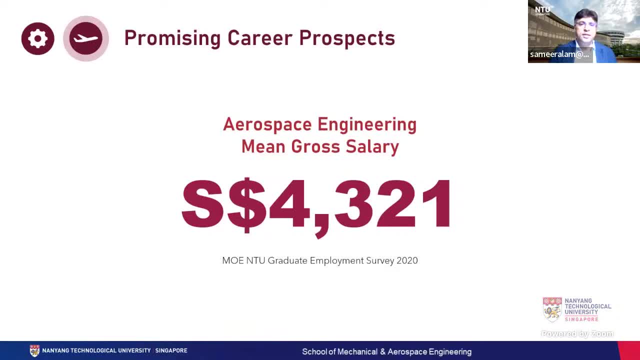 School of Mechanical and Aerospace Engineering. Mechanical and Aerospace Engineering also promise a very healthy career start. In the last year survey, the aerospace engineering mean gross salary was 4,321, which is a very healthy start. MA graduates also were able to diversify in various fields because of their cross-discipline. 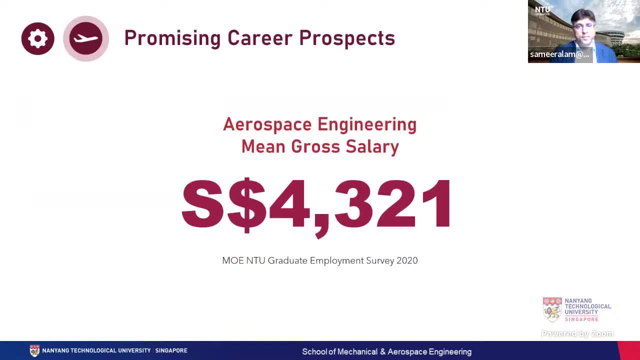 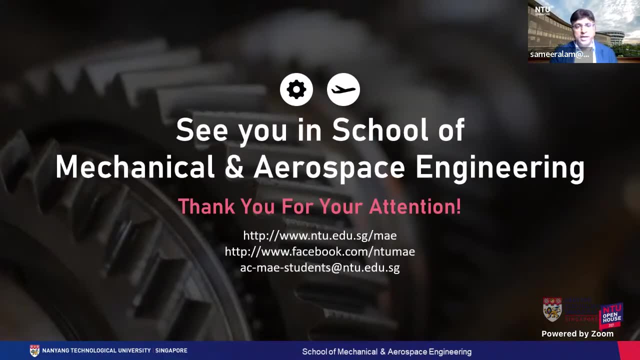 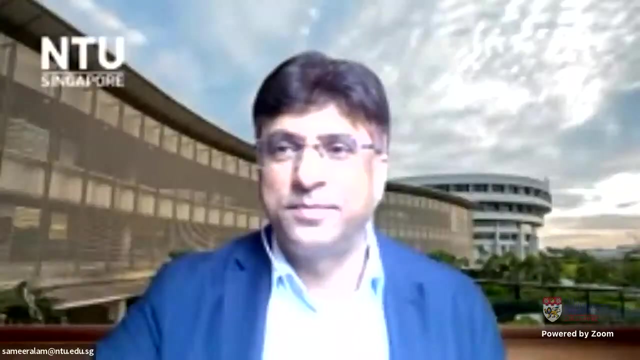 skills. So I would like you to invite to participate in this exciting journey in the School of Mechanical and Aerospace Engineering, and I hope that you are able to join us and propel the world forward as soon as possible. Thank you so much and thank you for your attention. 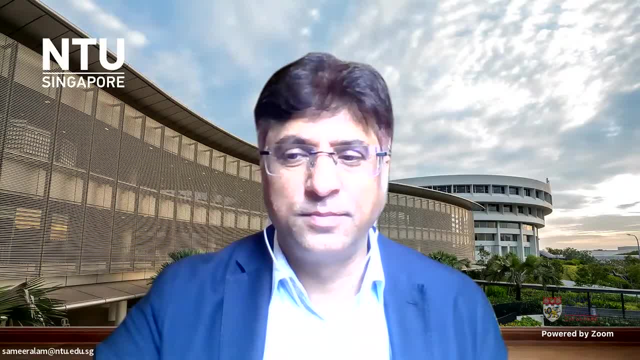 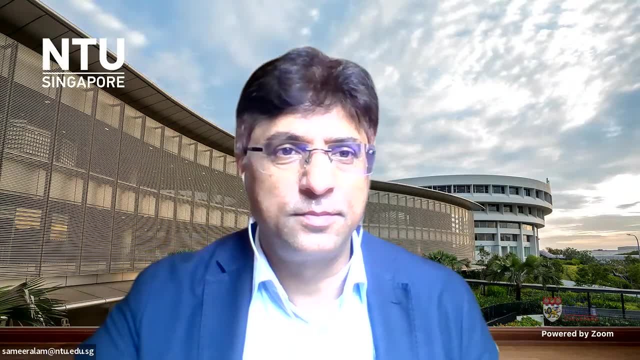 Thank you, Prof Samia. So now I'd like to invite Edna Edna from the Aerospace Society to share with you a bit more about what you can experience if you join the Society. So I recall about two years ago I actually helped the Society to get some discount tickets. 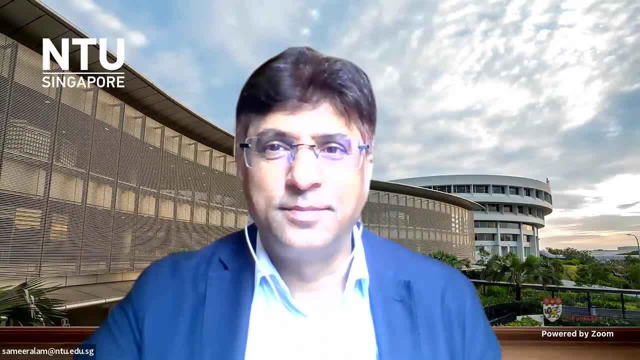 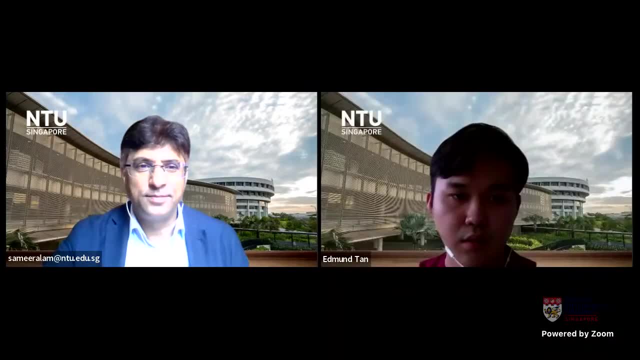 for the Singapore Airshow, and that's where I met Prof Samia again as well. So yeah, Edna, over to you. Okay, thank you so much, Eileen. Yeah, Hold on while I share my screen, Okay. 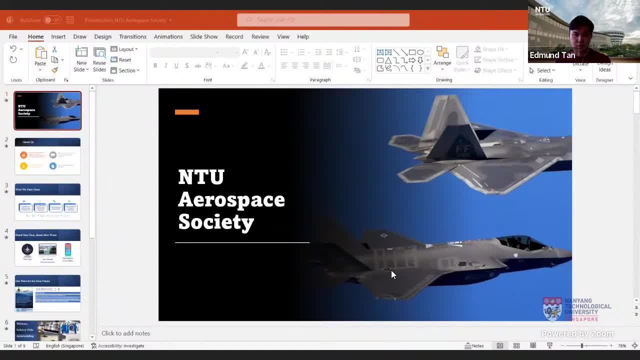 Okay, Hello everyone. So I'm Edman, the President of the NTU Aerospace Society. Today we'll be going through what the Society is about, what it has to offer and how it goes hand in hand with the MA module that Prof Samia has just introduced to you. 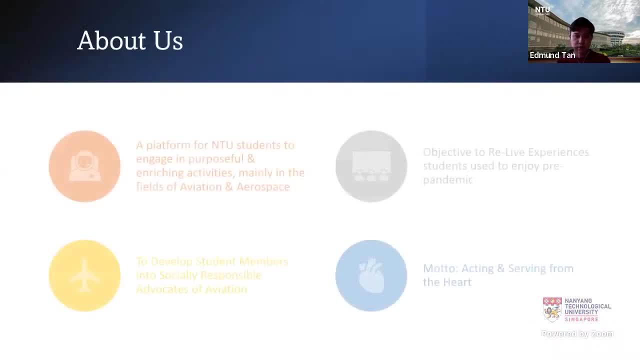 So about us? we aim and are a platform for NTU students to engage in purposeful and averaging activities, Mainly in the fields of aviation and aerospace. So this is so as to better pair and link what you have learned in school into the real life. 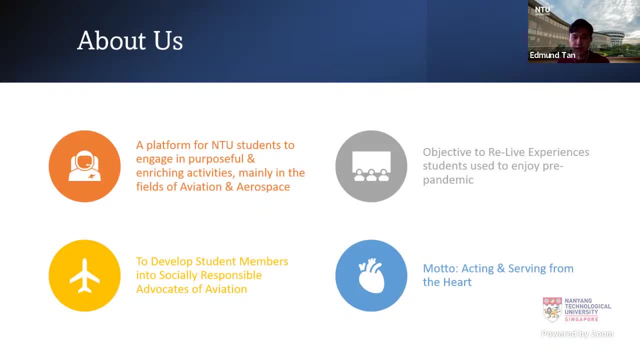 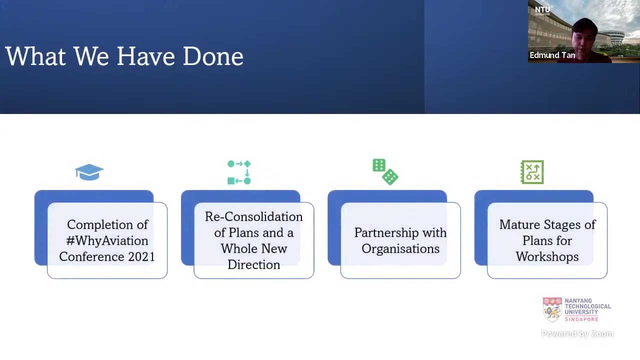 industrial practices and all right. We aim to develop student members into socially responsible advocates of aviation through our programs and we aim to relieve events that NTU students used to enjoy pre-pandemic. So what we have done so far Just the start of academic year 2021. last year, we have completed an online Y-Aviation. 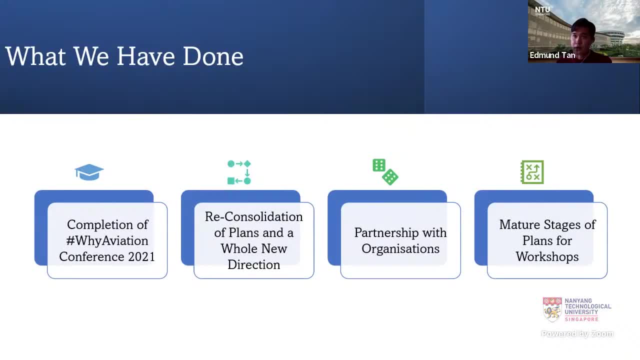 conference where we held a fully online event where we brought together people and leaders from aviation and aerospace companies together to talk about aviation trends, challenges in aerospace engineering and things like that. As a club, we have reconsolidated plans and aimed for a whole new direction where we take. 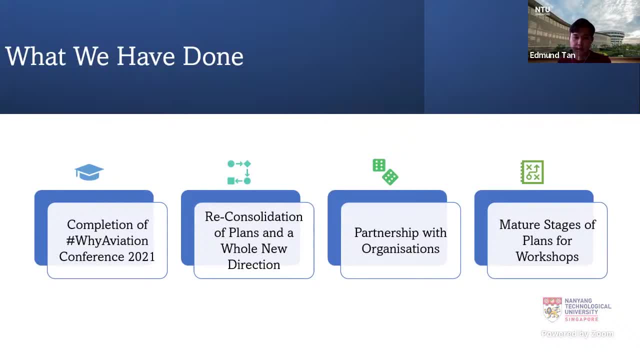 on more projects and plan more events for the betterment of all students in MA. We are partnering with organizations, two of which notable ones are the Singapore Institute of Aerospace Engineers and the Association of Aerospace Industries of Singapore, And we have also reached quite a mature stage of planning our workshops, which will tentatively 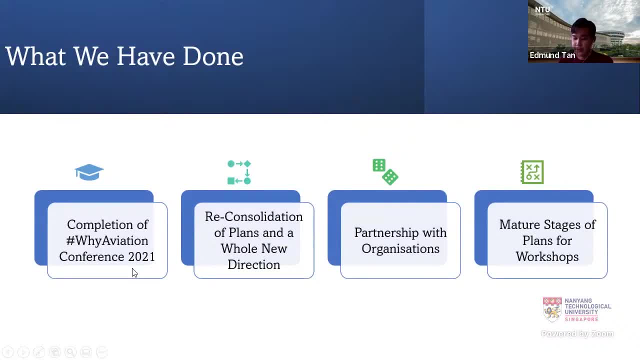 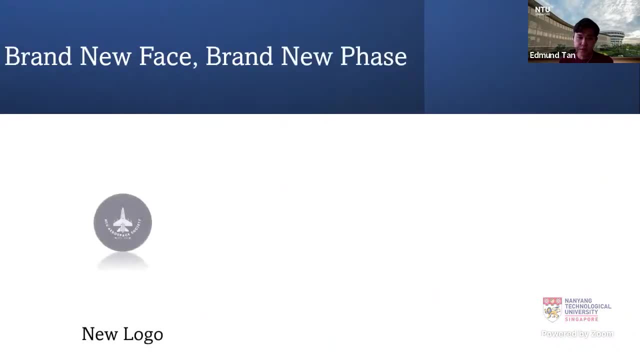 happen in June and July period or during the summer break. We are expanding our team to over a year. We are expanding our team to over a year. We are expanding our team to over a year. roller skill to accommodate to the new plans that we have. 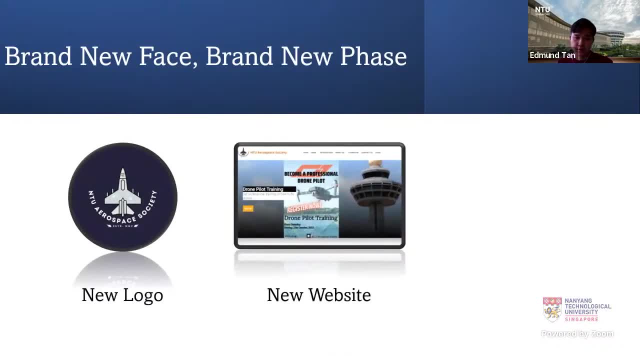 We have sought for a brand new phase and a brand new journey, with a new logo website which you can access though the hyperlink, or I will give you a QR code later at the end of the presentation. We have also a new phase for our main, our former social media platforms, which is the. 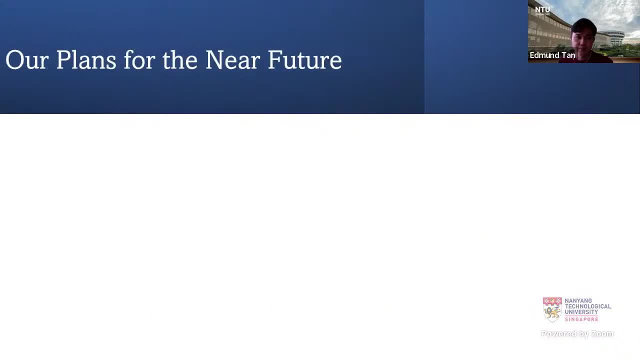 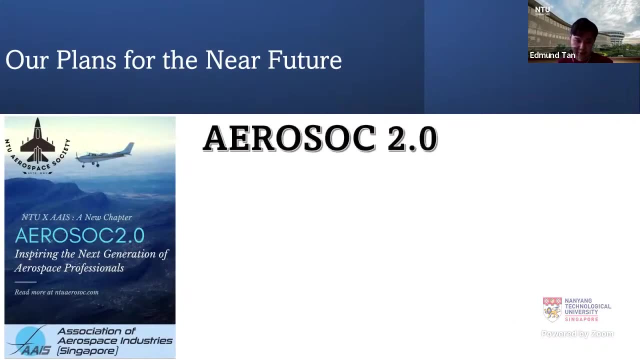 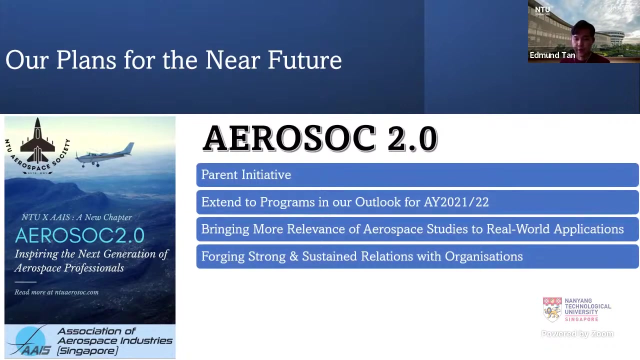 LinkedIn, social Instagram, Facebook and the Internet. So our plans for the future. Aeroscope 2.0 is actually a student innovation chapter initiative that came from the current committee right. it's looking to extend to programs. in our outlook for this academic year and even the next academic year we are bringing more relevance of. 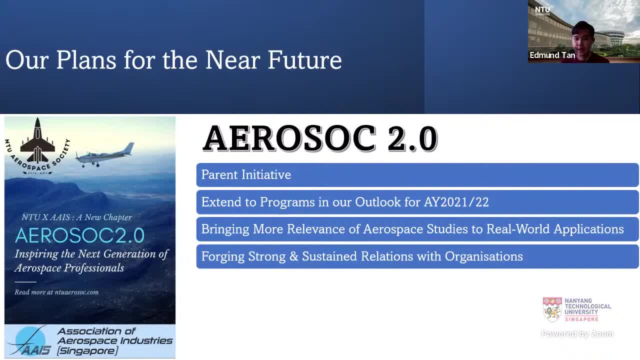 aerospace studies to real world applications and trying to bridge the gap between what students learn and what industrial leaders are looking for. so to do this, we have forged strong and sustained relations with organizations, as seen here. we aerosol 2.0 came as an initiative with 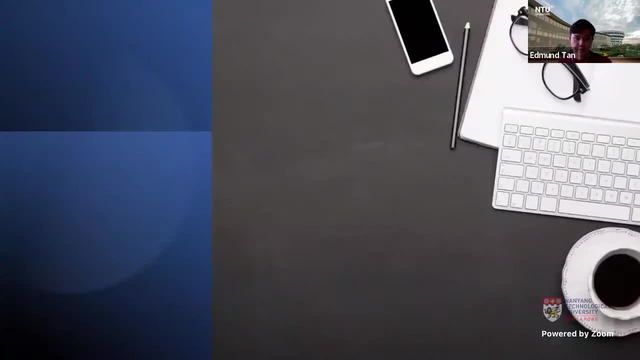 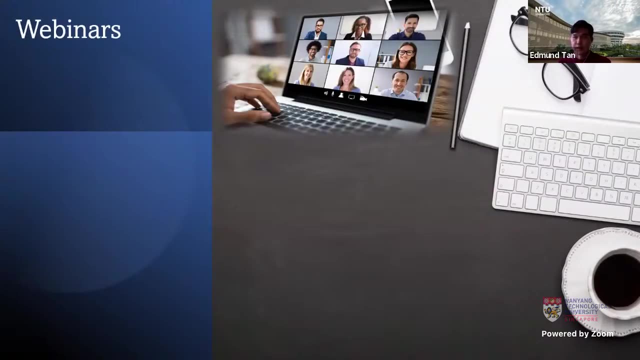 the association of aerospace industry singapore. so our plans for the academic year and the upcoming one. we have webinars. examples of webinars that we have conducted, uh are the ones with zara, if you know of her, the first female to travel in a single singapore aircraft. 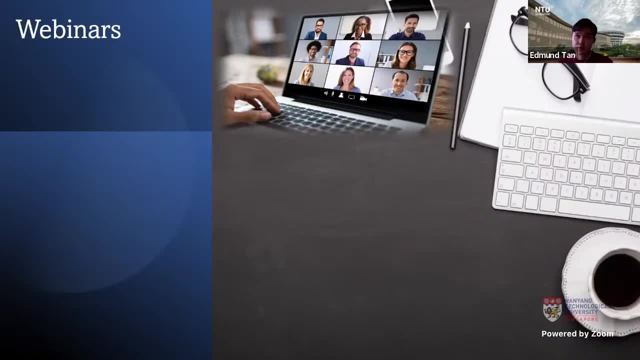 we have also just concluded a singapore aerospace technology and engineering conference with singapore institute of aerospace engineers. actually, this just happened, um, on the 16th of february, the most recent wednesday, and interesting enough, uh, like prof samir has introduced just now. right, the possible focus areas in collaboration includes internet of things, additive manufacturing and. 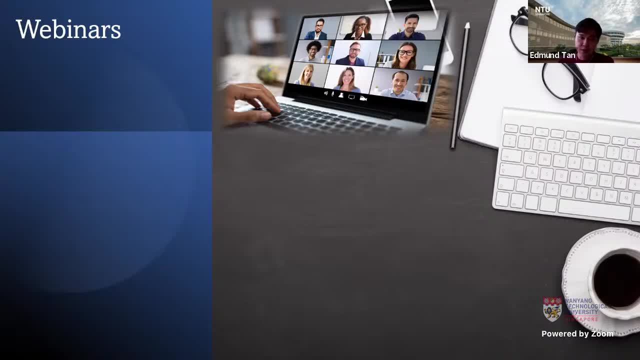 industry 4.0 and the topics that were covered in the most recent ítulo, La treballada de"-Singapurna era strangers and engineering conferences were actually updated as well. so we had industrial leaders, boeing defense, fa, we had french air force and the singapore republic of singapore efforts to come together and talk about that. 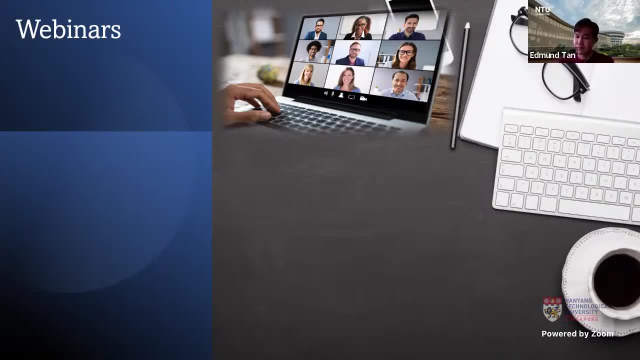 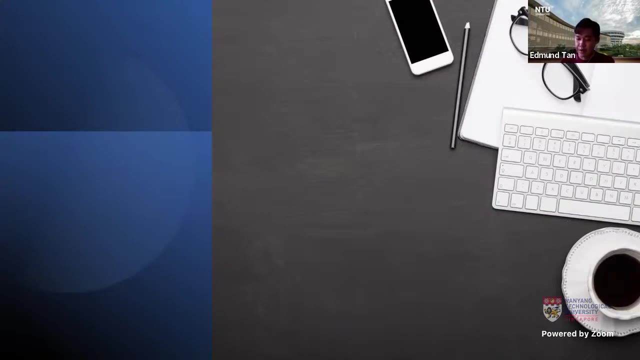 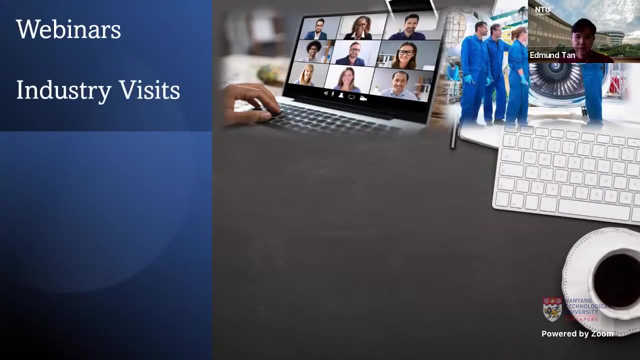 the trends, uh, that they are heading towards. uh, they have things like sustainability in aerospace engineering. what, uh, what business models they might have to to to, to hit in the direction. We have, fourth, IR technology, and we also have how data science and data analytics play a part in aerospace engineering in the industry. 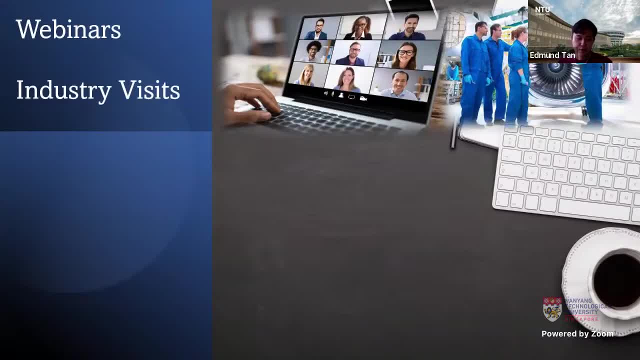 Next we have industry visits. This one is still in planning and we are looking to have our first one with Pratt & Whitney. In fact, Pratt & Whitney has reached out to us and said that they would want to head over to our school, NTU, to pay a visit to the students of MAE to share more about their 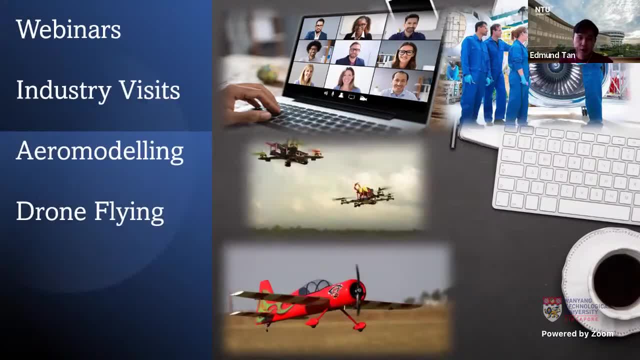 experience. Next thing: aeromodelling and drone flying. Drone flying, we had our first phase and our first trial run at the end of last year, December, So this goes alongside the plans that some students might have for their FYP. 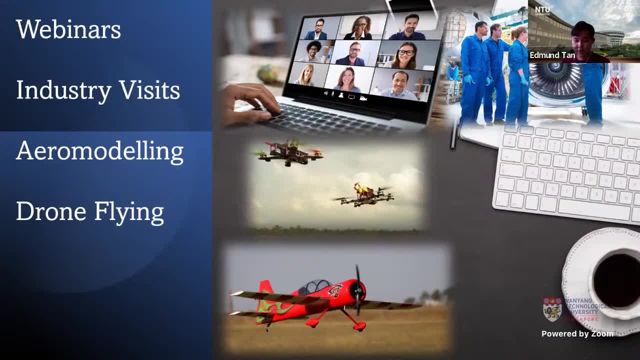 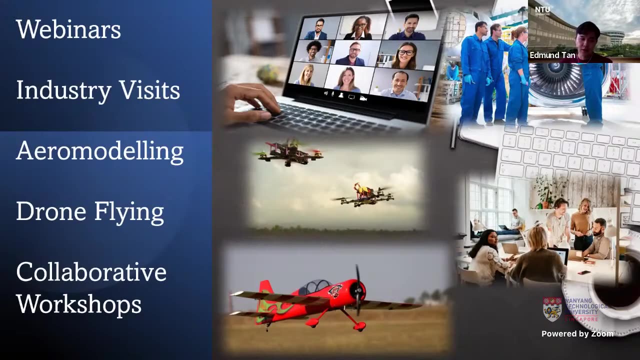 So, from what I've heard from professors of MAE, some students are looking to test their drones and all that. So we provide the training in drone flying and practice. Next, collaborative workshops. What I mean by collaborative workshops is even though you are in an anti-aerospace society. 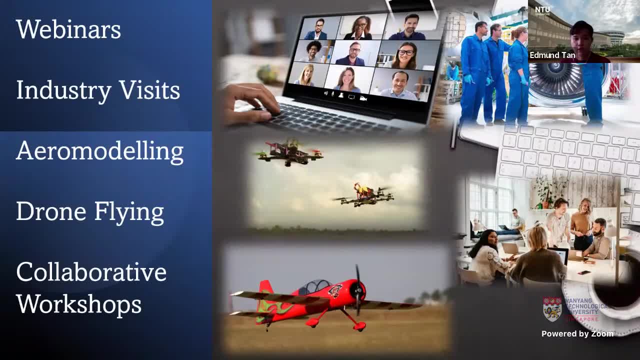 you get to experience activities that we hold alongside other clubs, For example LDP, which is also part of MAE, and we are looking to have our first one next Saturday. In fact, it's called the flight program, So we usually plan for this kind of collaborative workshops so that we can share information. 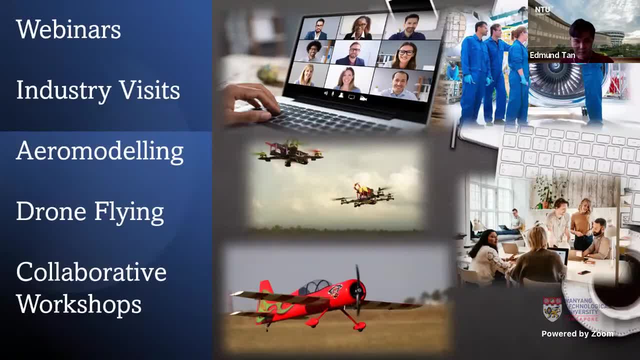 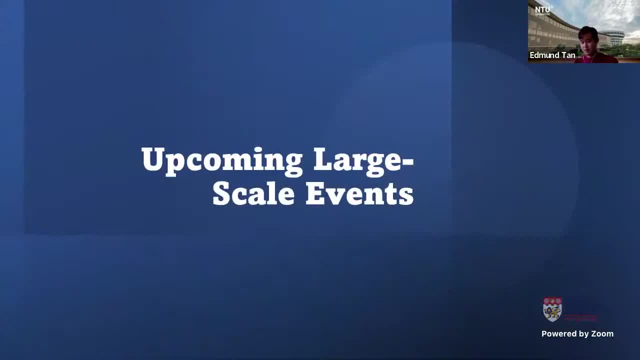 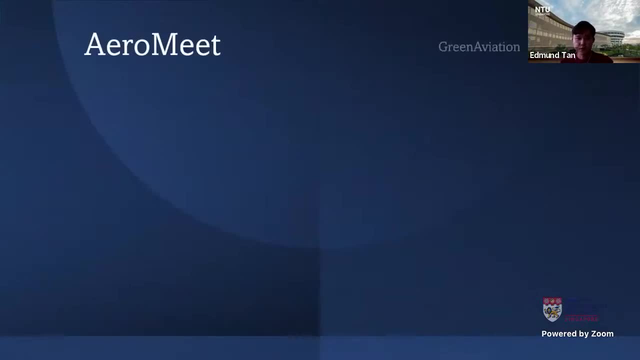 with each other, So we are from different clubs. Okay, Yup, and there's more. So to give you an example of two large scale events that we are currently in planning, you might just want to keep an eye out for these two: Aeromid and Green Aviation. 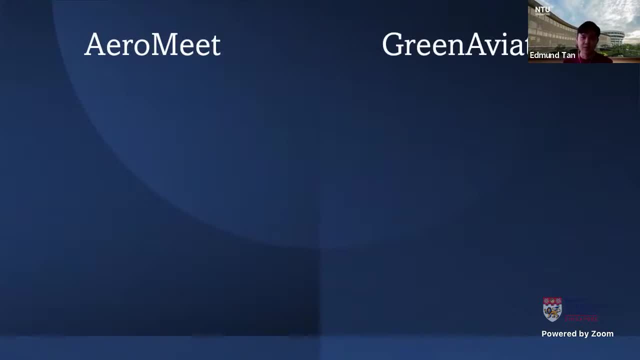 So these two are relatively large scale and we are still in planning with the organization Singapore Institute of Aerospace Engineers and also the Association of Aerospace Engineers. Okay, So these two right will involve a lot of major players in the aerospace industries. 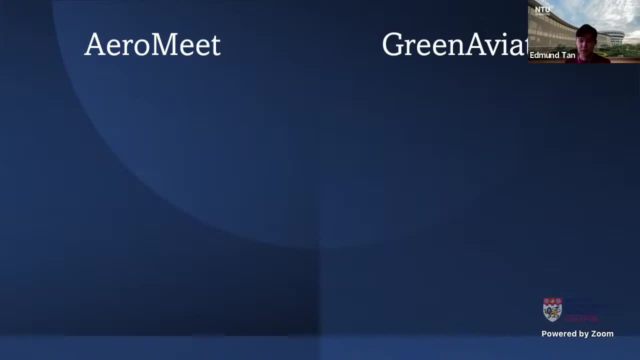 Yup, still work in progress And yup, Okay, That's the end of my presentation. Thank you so much. So if you all have your phones with you, you can actually use our QR code to scan this and it will be directed to our anti-aerospace society website. 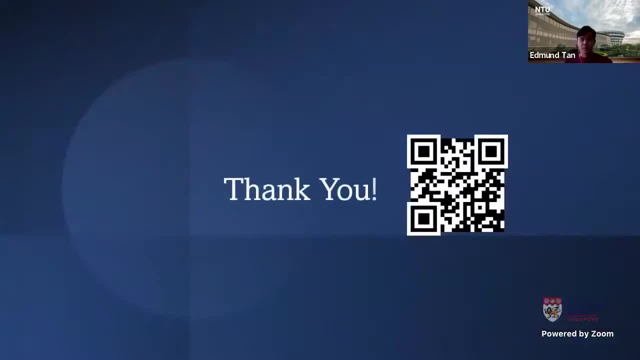 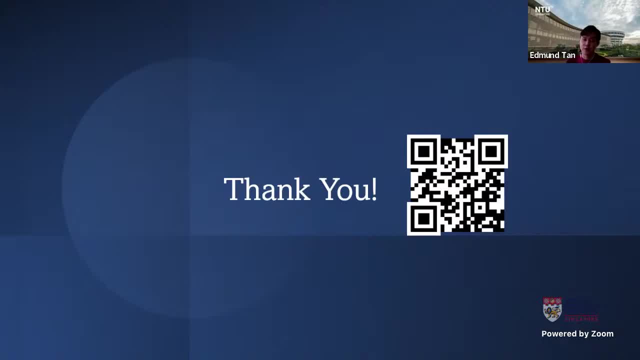 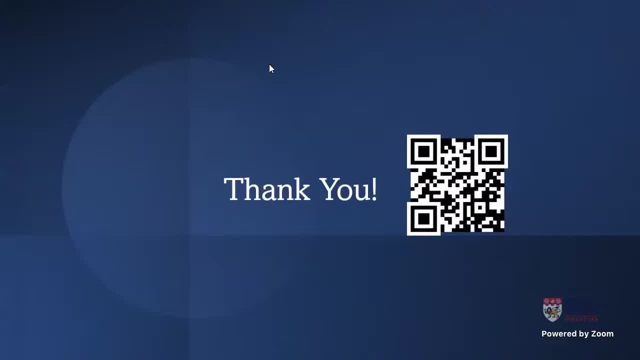 Thank you. Okay, thank you so much. Thank you, Edmon. So now the floor is open to questions. We have audience both on Zoom and on YouTube Live, so feel free to keep the questions coming in on either platform and I will forward them over to Prof. Samia and Edmon. 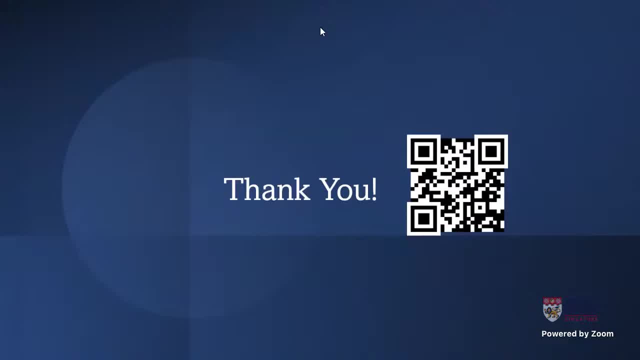 So now maybe, Prof Samia, in terms of undergraduate degree programme, do the students you know get to choose? are there, like some hands-on modules, where students get to, you know, either fix their own um mini drones, like what we saw on the screen just now, or are there any, like you know, hands-on? 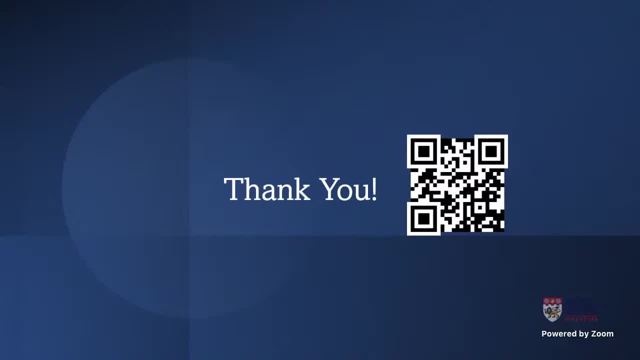 experience. i understand that we do have an air traffic management research institute on campus and one of the modules are actually um expose students to that particular lab. is that true? yes, elene, actually there are two modules, the two modules which students can take to broaden their horizon beyond, uh, aerospace, which includes one is air traffic management and second is the. 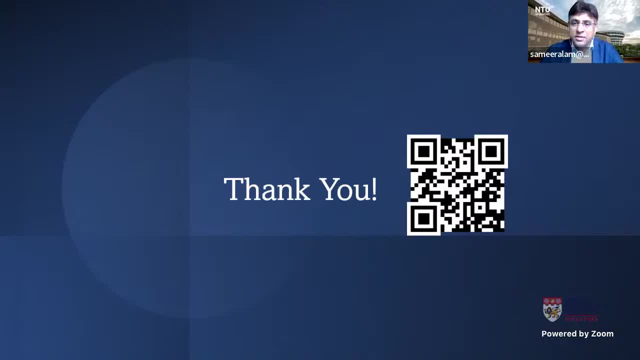 airport operations. so the air traffic management research institute has launched this specialized course two years ago for the students to give them a first-hand exposure of what air traffic management is. here, because of the simulation capabilities that we have in ntu mae, we provide students with hands-on training about air traffic. 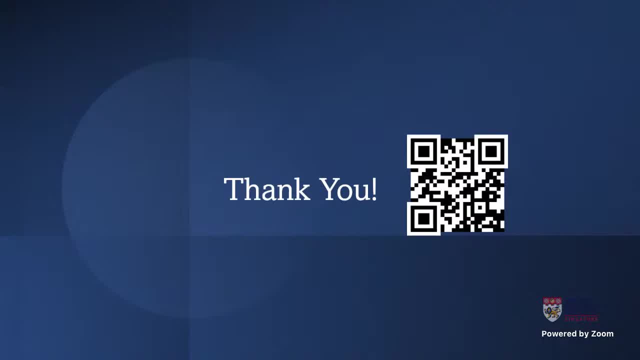 management, communication, navigation, surveillance, environmental impact of aviation. also how the airspace are designed, flight planning is done, so they look a very broader issue when it comes to air traffic management. they also participates in real world projects where they are given real world case studies about how the airspace can be optimized using artificial intelligence and 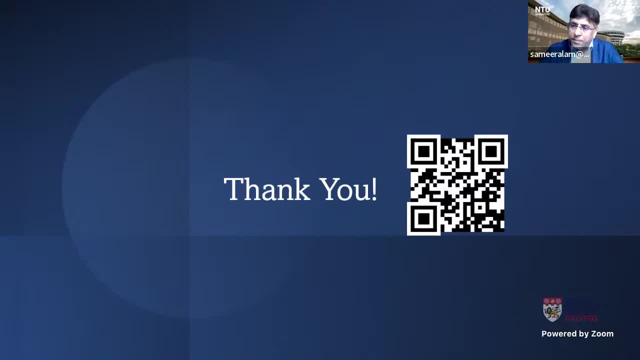 machine learning techniques. in the other course, which is about airport operations, students are exposed to various technologies and methods are for optimizing and airport operations, including terminal building design, runway optimization, taxiway modeling. all these things are exposed to the students which give them a very broad horizon of what aerospace engineering is. aerospace engineering. 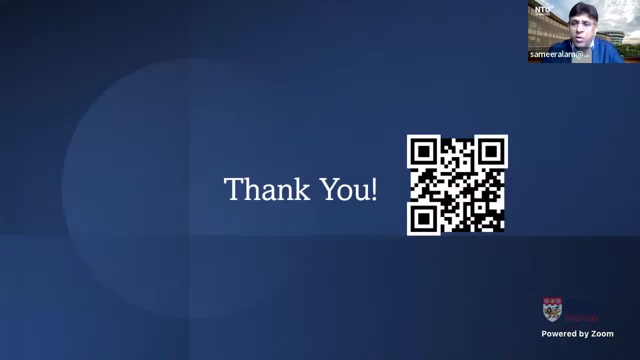 is not just about engines. try to understand this. it is about the entire air transportation industry. we aerospace engineers contribute to a wide dimension, so we should not think or narrow our vision when we talk about airspace engineering. aerospace engineers move the world, both in terms of airplanes and the system that enables this aircraft movements- ie. 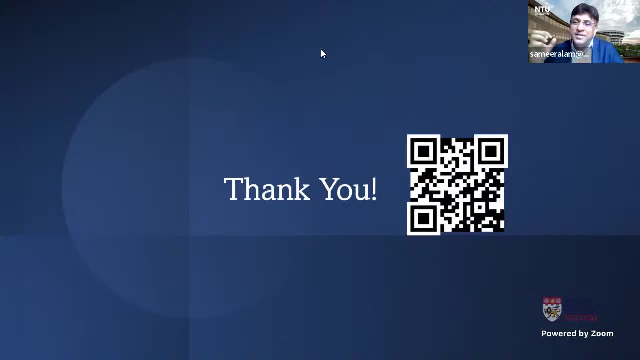 air transportation. also, the enabler entities in the system, such as airports, metrology, military air traffic controls- All these are the important ingredients of this air transportation network. So with this facility, I think students are very well equipped to explore the world and conquer it when it comes to the aviation. 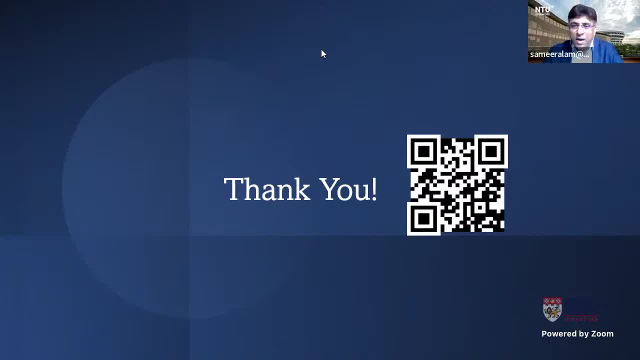 We have seen our students joining the Changi Airport Group doing airport operations, joining CAS doing air traffic control and air traffic management, or even going for their master's and PhDs in world-class universities in the area of aerospace, using AI and machine learning. 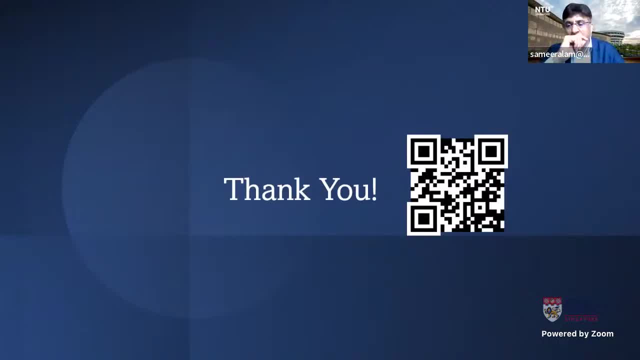 So this is a very unique school. Let me elaborate a little bit more on this. Other schools can teach about AI and machine learning, but we not only teach about AI and machine learning, but how to use them to solve aviation problems. This is very unique, very unique about our school. 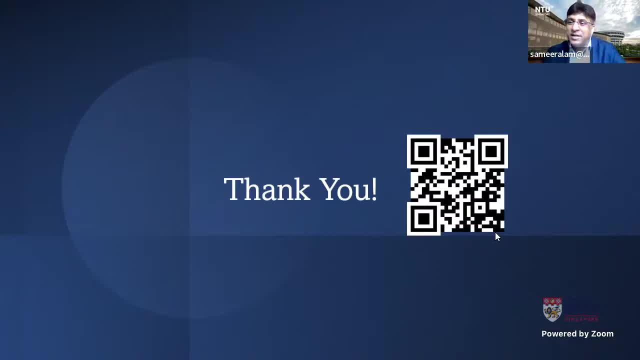 So we train not only students in aerospace engineering, But also about computational intelligence, computational thinking, Python programming, data science, artificial intelligence, machine learning. All these courses are part of AI, of aerospace engineering program. I teach data science and artificial intelligence. 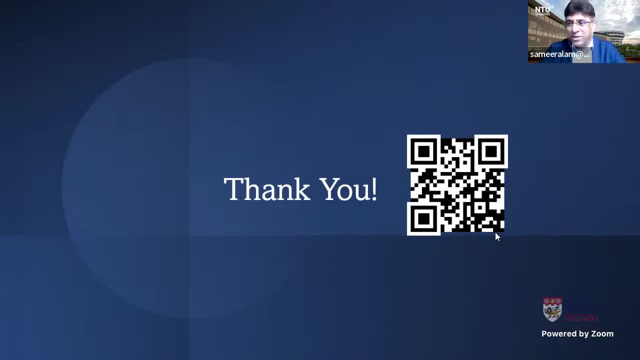 I also teach air traffic management, I also teach airport operations, So I can see how all those things can be brought together to give an experience to the students which is unparalleled anywhere in the school. Thank you, Aline. Thank you, Prof Samia. 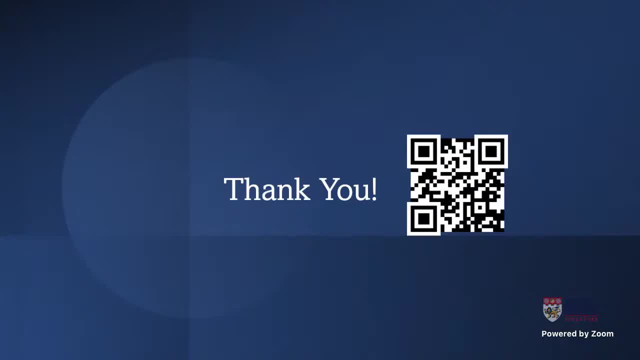 Okay, so I do have another question here. So, now that you know, with all these COVID situations- and we do know that the aerospace industry they were impacted in the past couple of years, But where do you see in terms of career prospects, which I feel that a lot of our undergraduate students, prospective students, 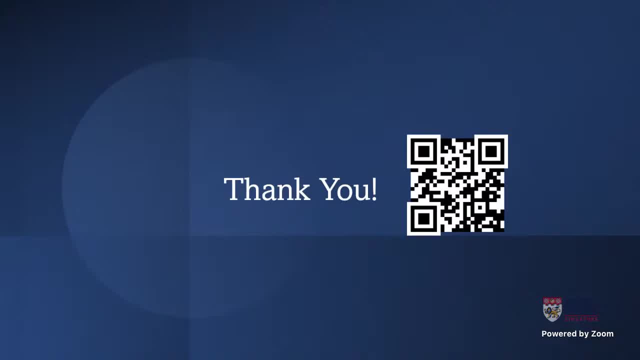 may be wondering about their career prospects When they graduate. graduate from this, so where? um? what do you think about the career market for aerospace engineers? in singapore? there is a metamorphic transformation for aerospace engineering industry. let me tell you how. general electric, one of the biggest engine manufacturing companies in the world. they have a 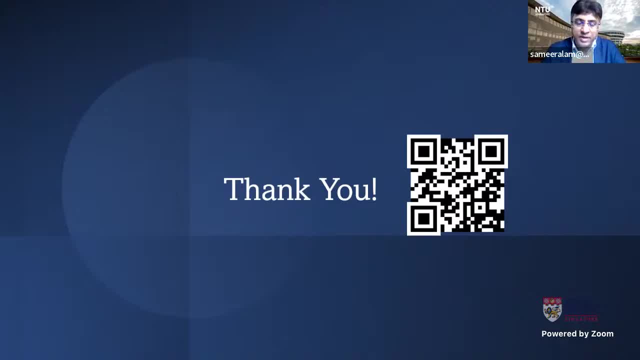 big plant and and facilities in singapore. they have just announced they want to hire 400 aerospace engineers because the backlog that they have developed with the opening of the aviation market is unprecedented. previously they were getting five engines per month during the covid time. now they are getting 35 engines per month, can you believe it? and they cannot service them. 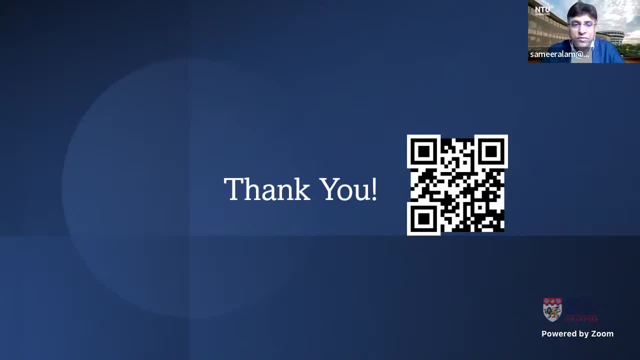 they need over 400 trained workforce for from from aerospace engineers to handle it. so next four years actually are going to be very exciting, as world has started to open and this is a time when young engineers, aerospace engineers who are trained in world-class institution like the school of mechanical aerospace engineering, can contribute to that. 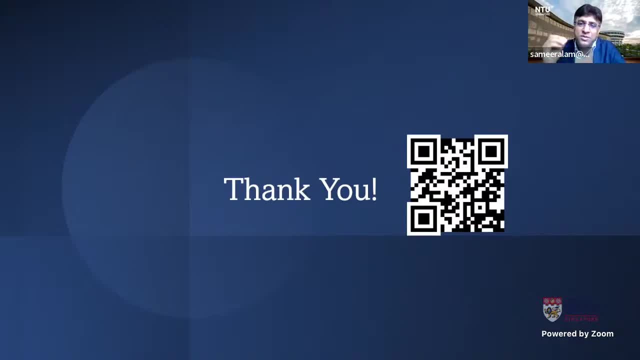 so next four, five years are very exciting. see, aviation is was the the most impacted industry because of the covid 19 and it will be the most rebounding industry after the covid 19.. the amount of excitement that is being building upon after the opening of the economy world over in air travel transportation. 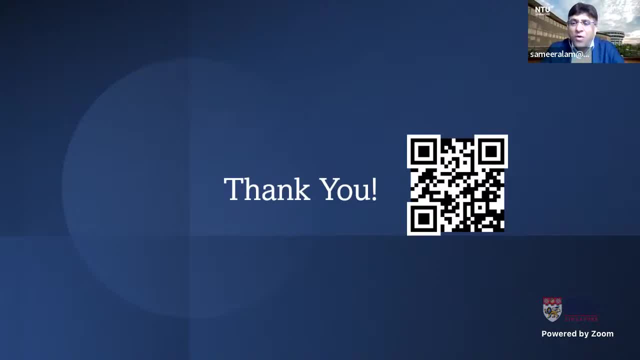 and people are getting back to normal. so you will see a surge of aviation activities, not only in in in air travel, but all the related engineerings, including mro, engine repair, overhaul, aerospace engineering, aircraft manufacturing. they all will be impacted positively. for example, airlines are giving big orders now, as we have seen in the air show, for new aircrafts because they 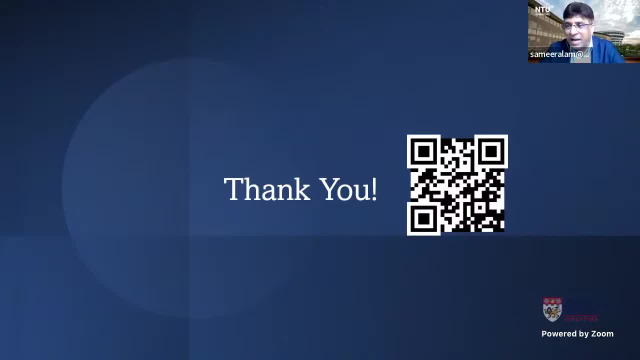 can see the tsunami of aviation travel coming again back, so this is the right time to become aviation aerospace engineers actually. thank you, thank you, uh, professor, i think um, just a second, um prof samia's um statements. right, we actually, i think recently i did see us a straight time article. 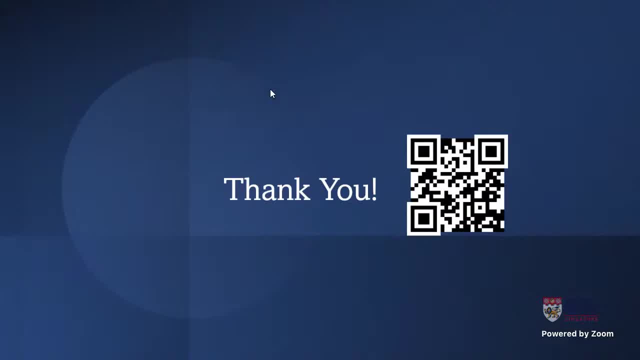 that actually states that you know quite a number of aviation aviation aircraft are getting back to normal. you know quite a number of aircraft are getting back to normal of the aerospace companies. they're expanding their hiring process. So you know, Prof. Samia. 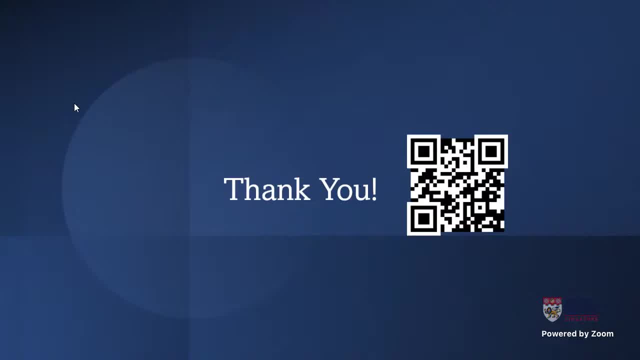 mentioned 400, and there were like companies like ST Engineering, Boeing, among others, that are actually, you know, looking to expand their workforce. So another question we have coming in. Some of our students would like to know if. let me see here. do they get to design aircraft when they're studying aerospace engineering? Of course, they learn the aircraft design. Aircraft design is a very important module during this course and they make use of advanced simulation, modeling and fabrication software to develop the various aircraft design We have. 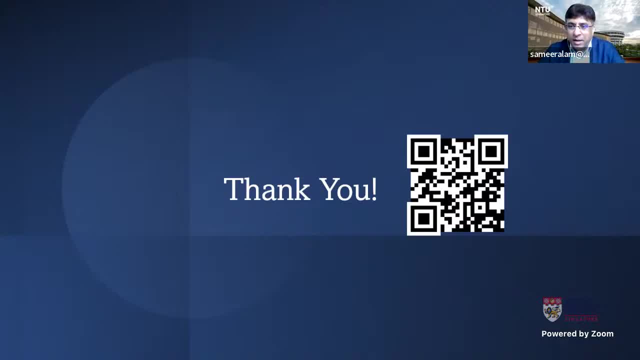 one of the world's largest air tunnel air-wind turbine right. So there they can test their various design when it comes to the wind tunnel modeling and can evaluate it. So a student not only get to design but also to simulate and evaluate. 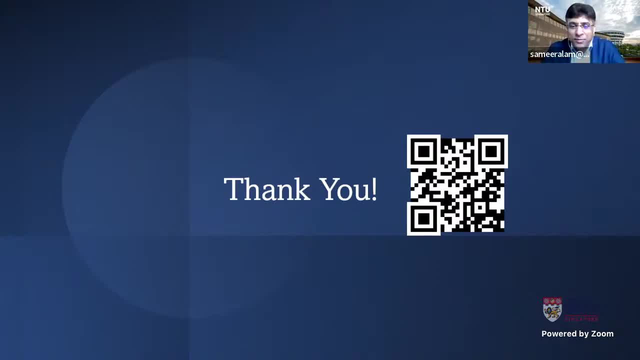 their designs, So they have. in terms of infrastructure, I would say: see, I have worked in Australia. I was a professor in Australia before. I have worked in France, in Middle East. None of the universities over there has the capabilities. 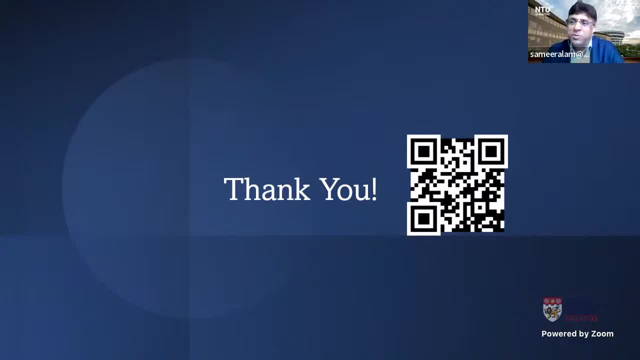 that NTU MAE has when it comes to the aerospace engineering students. The infrastructure that we have allows the creativity of the students to take shape. They are able to see the realization of what they want to do. Our school provides them, So they are not only to do. 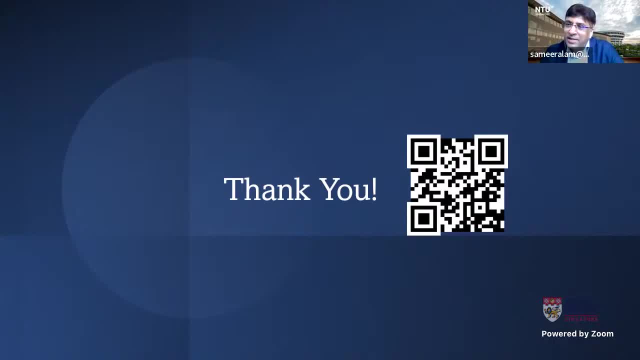 aircraft design, but also to evaluate, simulate and fabricate, and to test also. No other university allows the students to have this kind of experience, from the idea what they have to the realization of the product they have. Thank you, Thank you, Alin. 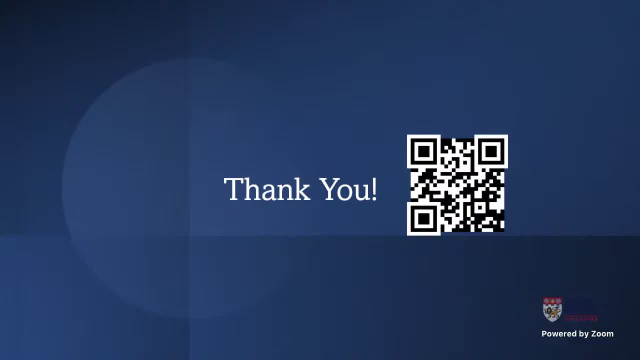 Thank you, Prof Samia. Okay, let me just take a look on our Slido to see if there are any questions. Okay, so we do have a question coming in. What is the difference in roles between an aerospace engineer and an? 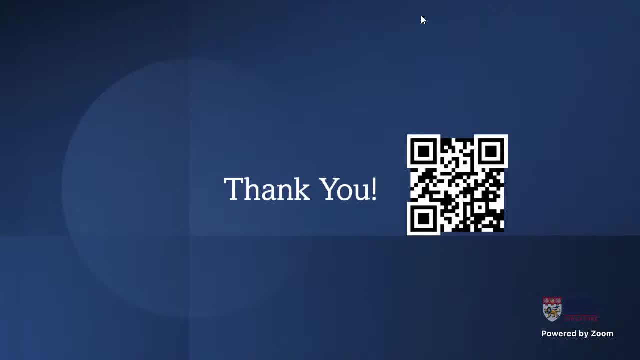 aerospace diploma graduate in the industry. Do the employers Yep correct? Go ahead, Prof Samia. So we see, with aerospace engineering, students have a very in-depth study of the engineering aspect, which a diploma student may not have. 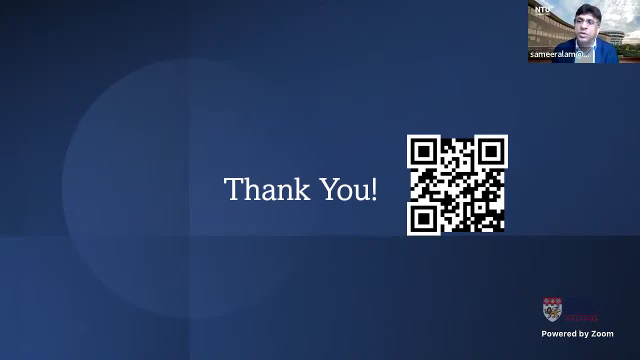 Also, the aerospace engineering students have a wider dimension when it comes to the aerospace engineering And a diploma engineer can only work on a certain aspect of aerospace engineering, Whereas a trained graduate engineer aerospace engineer has a variety of dimensions where they can go as a consultant. 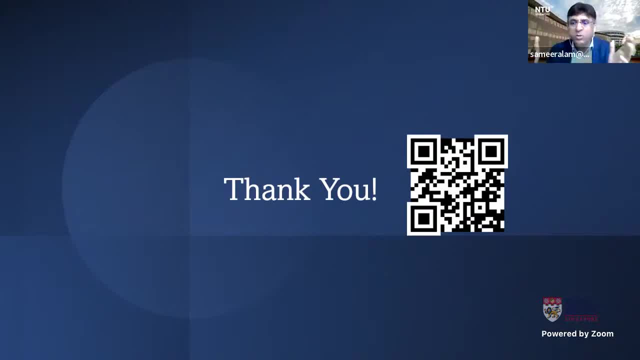 airport engineers, ATM experts- all those roles are open. So the job prospects of an aerospace engineer are far, far more than a diploma holder. So diploma holder, because of the nature of the study, they are more focused on a particular aspect. 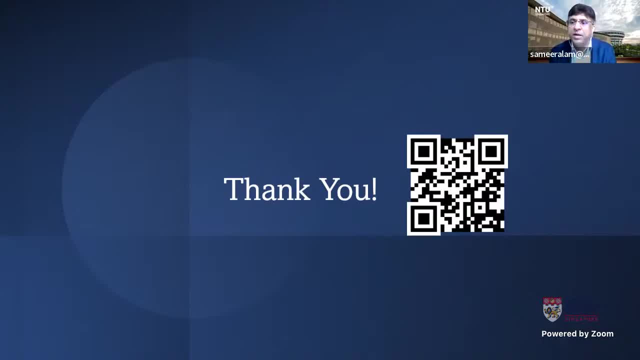 of aerospace engineering, Whereas aerospace engineers, by training, they experience and explore a more wide dimension when it comes to the aerospace industry, Also when it comes to the future career prospects, of course, in terms of career progression, when you have to. 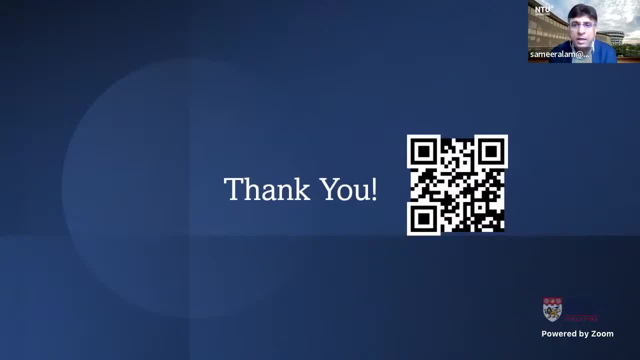 go to a higher management position. if you have a formal degree in aerospace engineering, it certainly helps. Now, maybe I would like to ask our audience in the Zoom platform if they have any questions, to drop them in the comment box. I have someone who dropped. 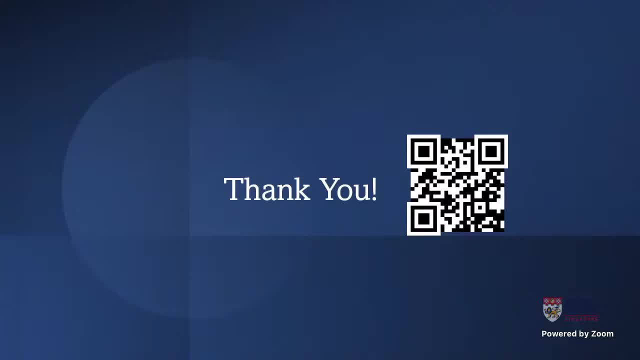 me a private message here. Can I ask the significance of Singapore as an emerging country in the aerospace industry? Do you have any thoughts on that? Prof Samir, Singapore is not an emerging country. It is an established country. Singapore is very well established when it comes to. 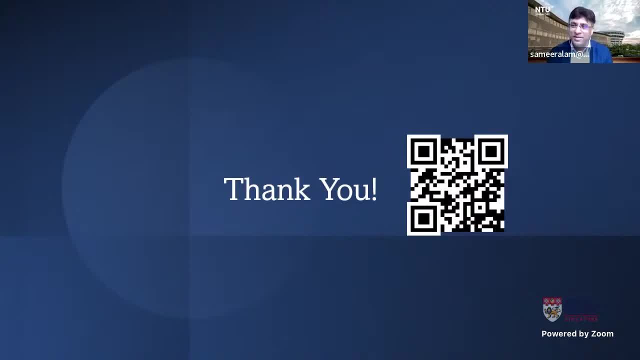 the aerospace. We have world-class airport, World-class airport, Changi International Airport. We have a world-class airline, Singapore International Airline right. Our air navigation service providers can be seen as a world leader when it comes to the forefront of advanced. 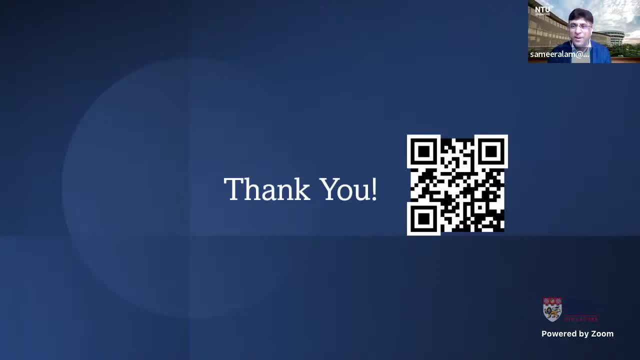 communication, navigation and surveillance facilities. So Singapore, in terms of aerospace, leads the world in all the dimensions. So it's not a new market, It is very well established And also there's a historical precedent to that. Singapore is on. 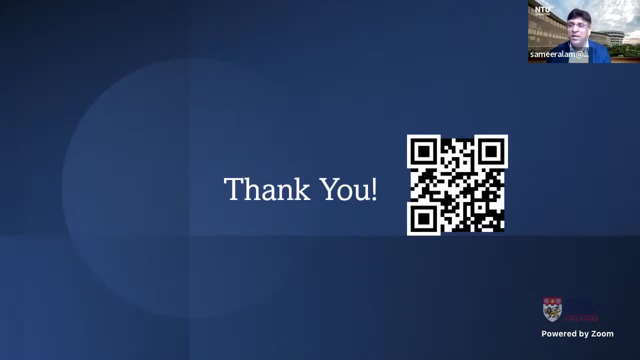 the- I should say- a trade route between the East and the West. It connects East and the West. It's a link between East and the West, So we have a geographical advantage as well. We connect the two worlds. Singapore is an enabler, And that enabler 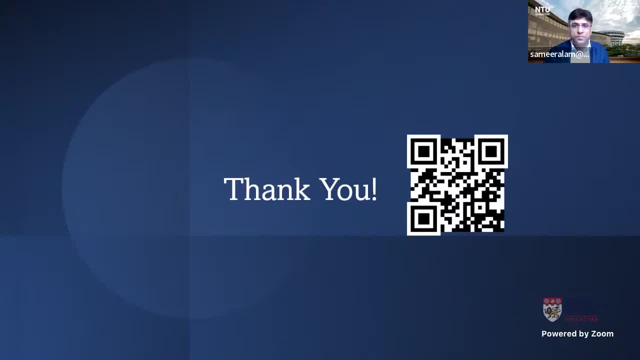 catalyst is the aerospace industry in Singapore. Okay, Coming in from our Zoom chat, there's a student who is asking: oh, there are two questions here. The first one is actually: if they study, what is the difference if they specialize in aeronautical? 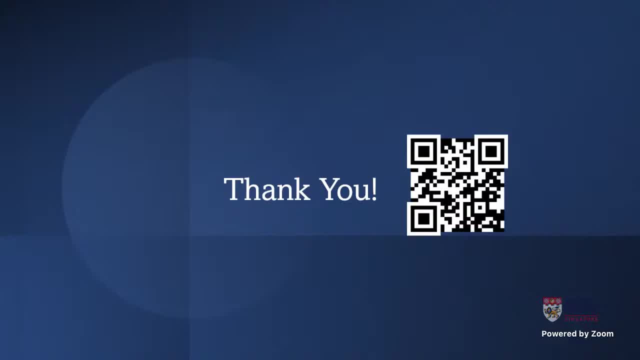 engineering versus a bachelor in aerospace engineering. Is there a difference if, let's say, eventually they graduate, they want to enter in an aviation industry? does it matter which, whether they take a specialization or whether they take a bachelor, Because in both of these degrees they do get exposure. 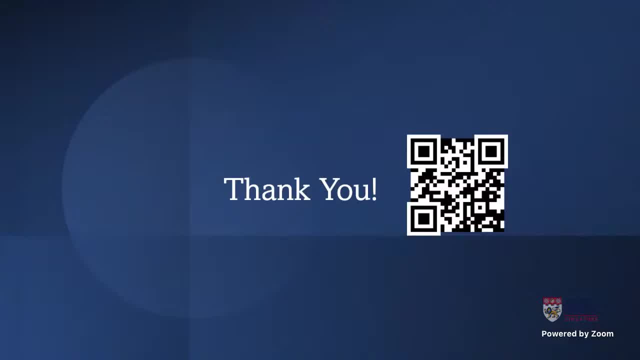 to the aerospace curriculum. Yeah, you're right, Eileen. Actually, NTU is one of those universities which allow students to have the flexibility to choose a wide variety of courses. So it doesn't matter what specialization you look for, We make sure that you are excellently. 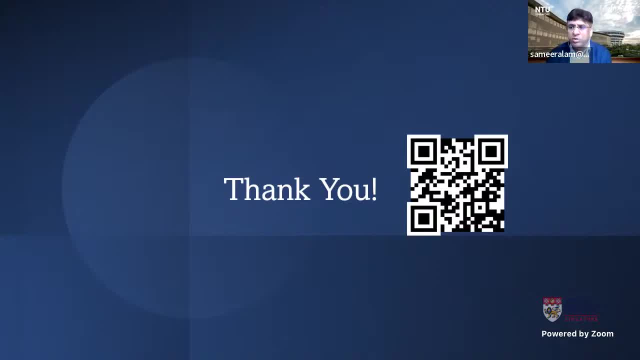 trained either in aeronautical engineering or aerospace engineering. The amount of exposure that you get is sufficient for you to understand both the dimensions, So do not worry about specialization now. Once you will come into the school, you will be seeing lots of. 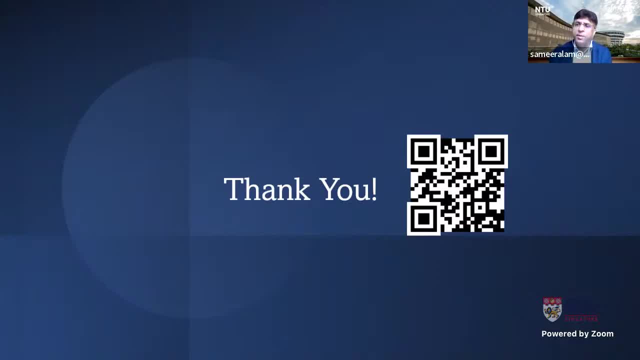 possibilities. You will be able to decide yourself which particular specialization gives you more enriching experience. Different students have different likings. It doesn't matter which specialization do you go to, as long as it matches with your interest. If it matches with your interest, I'm. 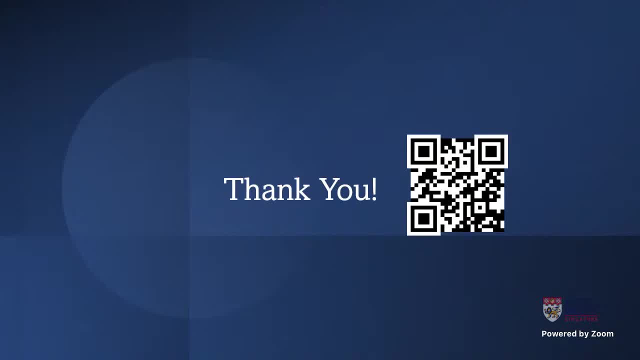 sure you are going to excel in that. Okay, However, Prof Samir, let's say I am a prospective student and I am interested in the aviation industry, but I can't decide if I want to specialize in it or if I want to take. a bachelor's degree, because I think they are quite different. One is under mechanical engineering with a specialization, whereas the other one is straight away. we start with the aerospace curriculum. So between the two, where do you think is the difference? If I study, for example, aerospace engineering bachelor's degree. does that give me an upper hand, for example, because right from the very first year we do have a lot of like you know, we start studying aerospace related modules- or would both give me an equal placement as compared? to my peer. See, it all depends upon how you like the courses right. If you have a mechanical band of mind, you will enjoy mechanical engineering more. If you have aerospace passion for aerospace, I would suggest you to go for the aerospace. 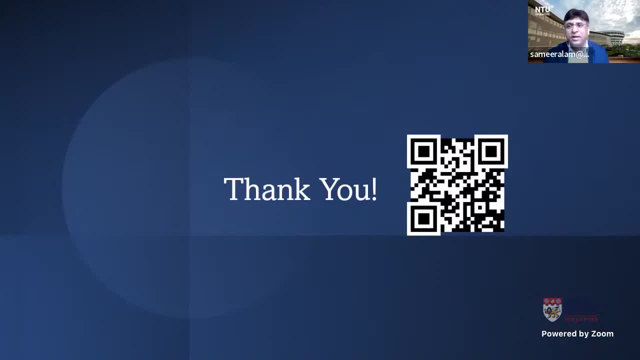 engineering. See, both of the experience are unique, right? It is not that one experience will give you an advantage over the other group, or one group will give you an early job prospects then. So there are so much soft dimension of your personality that 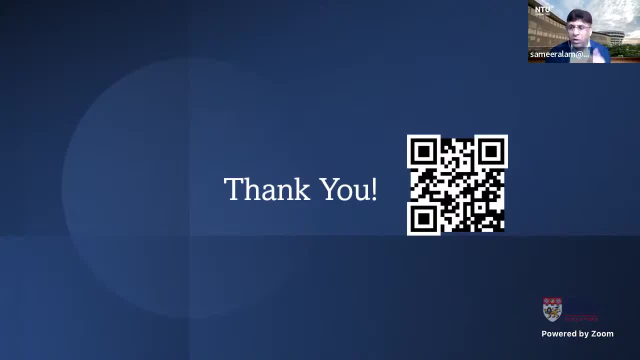 decides how you ace a particular interview. If you are a good engineer, if you have a good presenter, if you have aced your modules very well, if you have a high distinction, you will be able to make a mark in the industry. 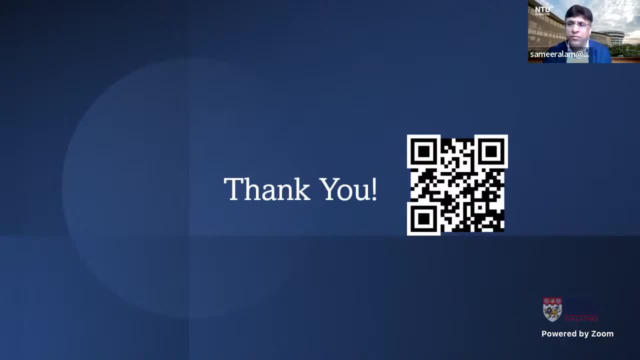 So in that sense, I would encourage you to choose either of one of them. I would say, from my prospect, if you start with a mechanical engineering which is very broad-based and you specialize in aerospace engineering, it's perfectly all right. And if you start focused with aerospace, 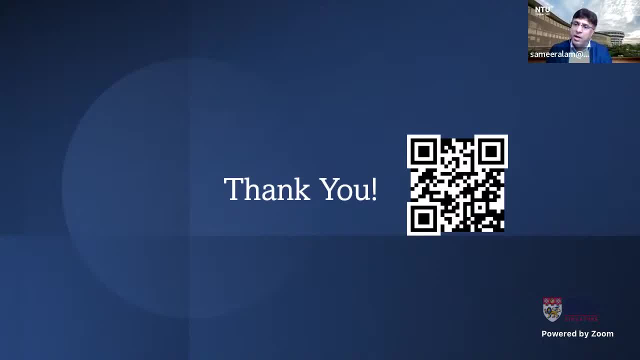 engineering. it's also fine because you will be exposed to other modules which are related to mechanical engineering one way or the other. So mechanical aerospace engineering. that's why the school has such a broad choice of the electives. These electives are when they come, these electives. 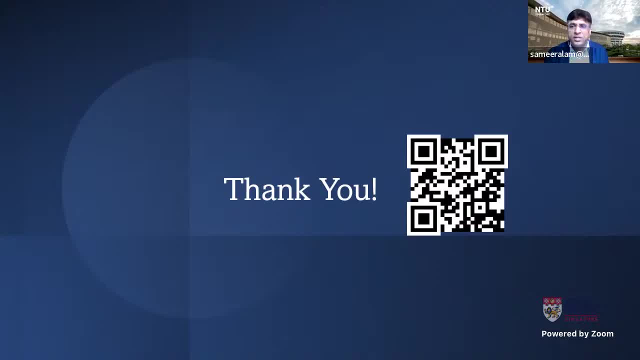 you will be able to make most of your passion, of what you want to do in the later. once you graduate. First year, second year, all the courses have a similar engineering flavor. What do you specialize in? You should focus when you come in third year. 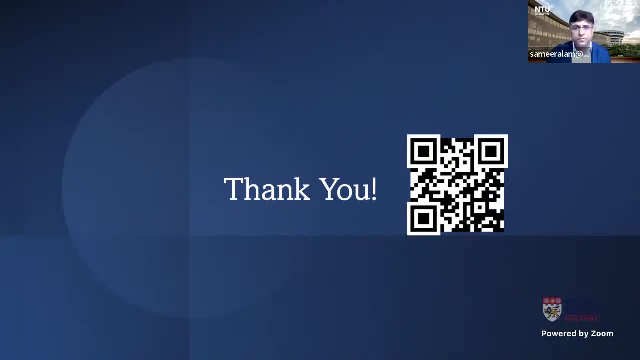 or fourth year, once you have a good understanding, Mimi, I can just add in an application tip for all the prospective students. So while I think both give you equal exposure and I think both has its own advantages, if let's say you. 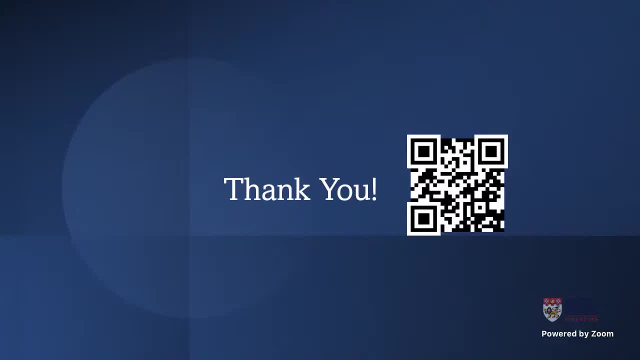 are undecided on which program you want to apply for, I would say if your cut-off point actually qualify, you can try for the aerospace engineering program as the first choice And the reason it's usually a bit easier for you to transfer from the aerospace. engineering program to the mechanical, as compared from the mechanical to transfer to an aerospace degree program. This is actually due to the supply and demand. So in the aerospace engineering program generally the cohort size is slightly smaller So it's a bit harder to get in. So, if you can, if your marks, can you know? if you can hit the cut-off point and you are undecided- that's only for people who are undecided yet- you can still put aerospace as your first choice And if, let's say, eventually you choose to go to mechanical, 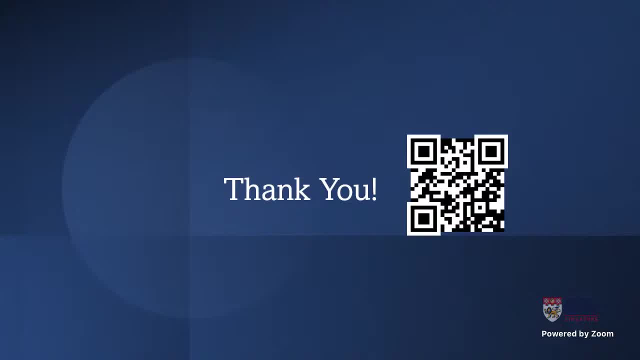 engineering. the option is always still open for you over there. So we have another student. We have two more questions on Zoom. The student is actually asking if is there a job security if you work in? let me see. is there a job security if you? 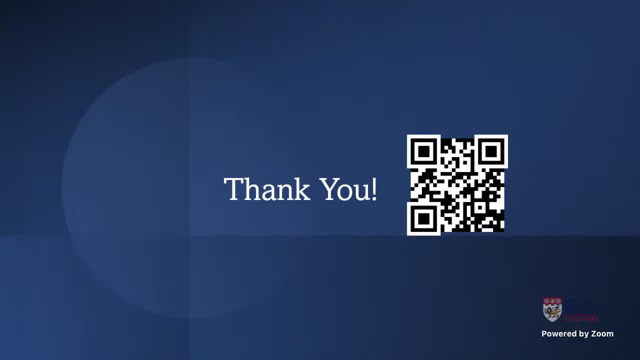 work in aerospace industry in case another outbreak or crisis happens? Prof Samir, what do you think of the job security in this aspect? Very interesting question. So see, the outbreak or crisis has not only impacted aerospace industry. it has impacted all the industry. 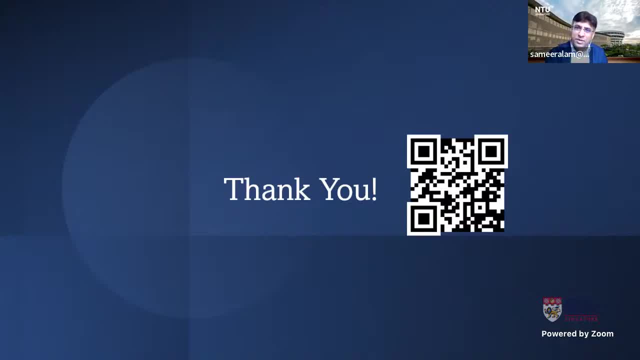 Right, Because we live in a global village where all the industries are interconnected. So if you are a pilot or an engineer or a technician or even civil engineer, if they are associated with the aviation, they got impacted. People in the hospitality industries, hotel industries. 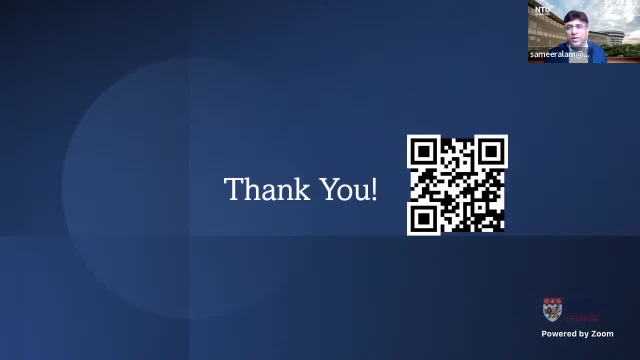 accountants over there. they got impacted. So this is the new world that we have to live into. We have to be adaptive and all when some crisis happens, all the industries get impacted. It's not just one industry got impacted, All the industries got impacted. 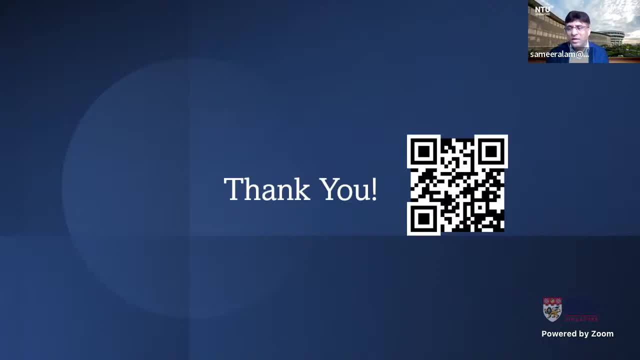 So we have to be resilient, We have to be prepared when such crisis happens. So I think engineers, in itself is our training to be resilient. So that's my take on that. Yeah, I would say that it's true, you know. 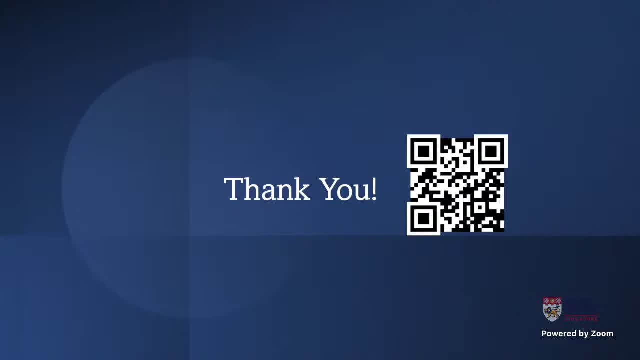 not just aerospace industry. actually I think across many industries the jobs are never. we can't really expect you know what can happen in the future. but what we can do is we can equip ourselves to be ready, to be resilient, to be 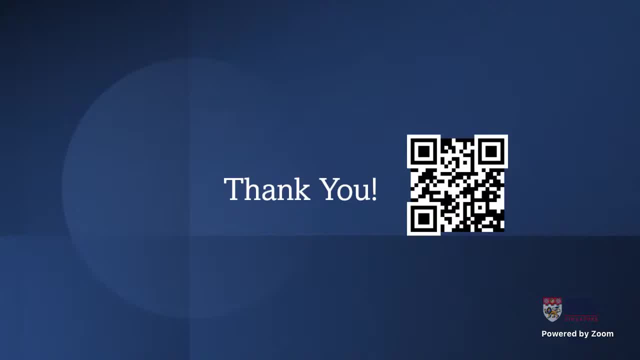 well equipped, you know, to adjust to different kind of prospective jobs in terms of different fields. I think, with the knowledge and the skills applied, we have seen many graduates actually not just excel in engineering, but they excel in many various fields, and that's because I 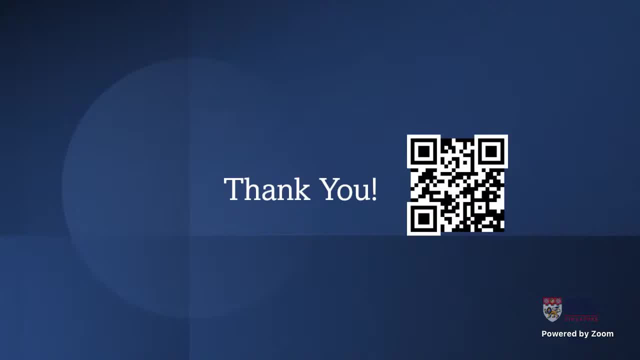 think with an engineering degree and also with our current curriculum, we do have that advantage of versatility, making you very versatile, making you very agile, making you very adaptable to different situations On here. okay, on Slido, we have a question. 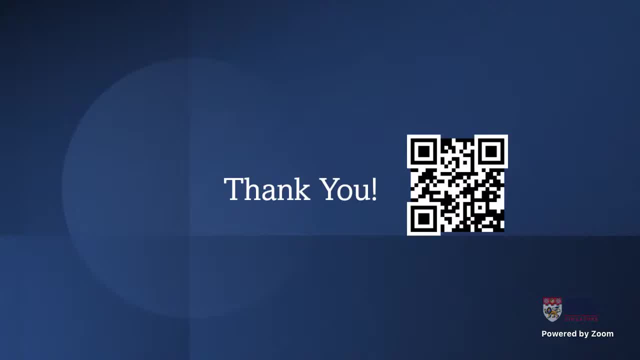 directed for Prof Samia. Once again, Prof Samia, very popular today. What do you have to say about um, the displacement with technological revolution in the aerospace industry? Very good question, actually very good question. Every time a new disruptive. 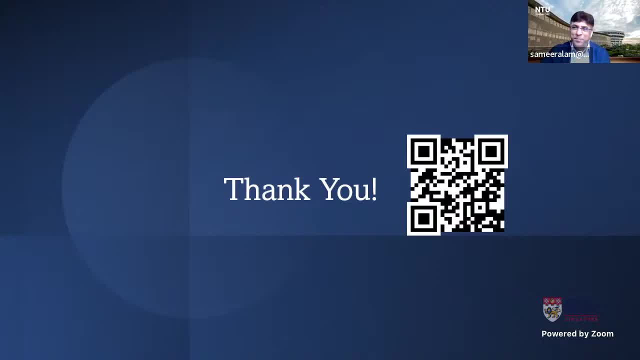 technology comes, it brings new opportunity. Before aviation industry kicked off in early 20s, the transportation was mainly the rail travel, and this disruptive technology at travel brought new opportunities. Now we are moving towards digitalization of aviation and air travel right. 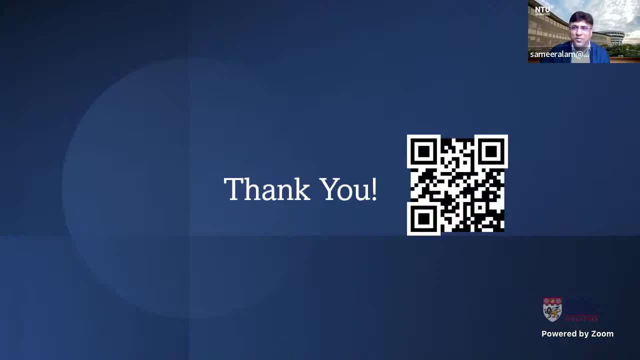 That's the reason that in the School of Mechanical Aerospace Engineering we have few courses that equip you to train you to be ready for this digitalization revolution that's happening in aerospace industry. We train the students in computational modeling. We train our students in programming. 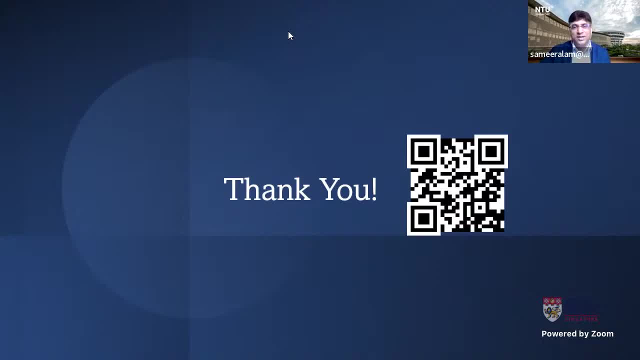 We train our students in data science and machine learning And we do several projects. Actually, the fourth profile of the students that I showed you before, they all are MAE undergraduate students. They excelled so much in their research. undergraduate research when it comes to aviation. 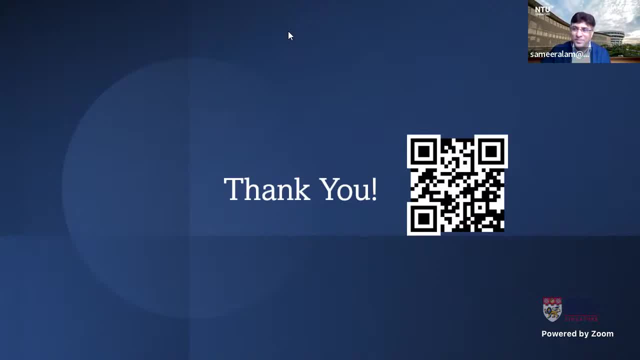 that their research was published in top journals of artificial intelligence and air transportation. So this is a realization of the change or the disruptive technology that we have in the School of Mechanical Aerospace Engineering, by equipping our students on these disruptive techniques So they are able to contribute. 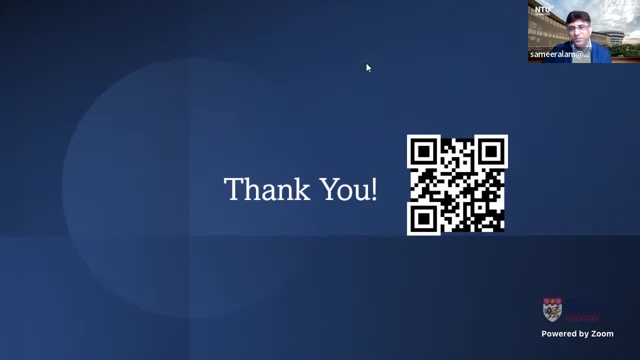 to the new generation of aviation that we are transitioning into. We have time for just one last question from Prof Samir. It's from Oslaido, So this student is actually asking: are your modules designed to also equip students with digital skills such as coding? 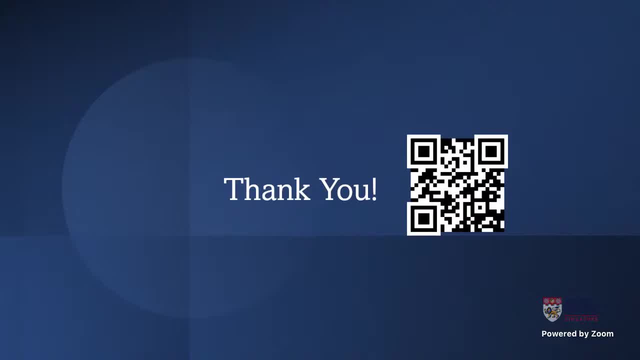 for example, considering the increasing demand of such skills and the changing nature of today's world? Oh yes, As I mentioned to you the courses that we have in the Mechanical Aerospace Engineering on data science and artificial intelligence, Python, programming, computational thinking. they equip you. 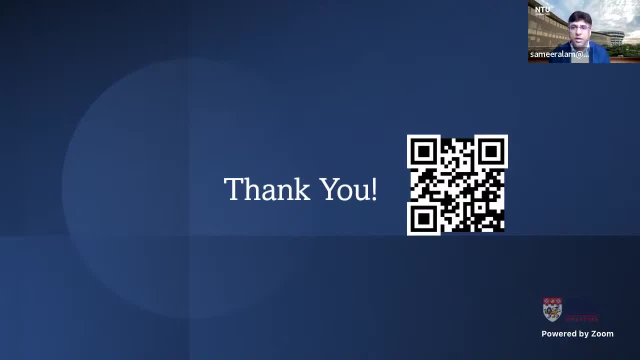 and they train you on programming skills. So we make sure, when you graduate from here, you are ready for these challenges If a job requirement requirements require you to be ready for the softer side of aviation, ie to be digitally knowledgeable using computational modeling and programming. 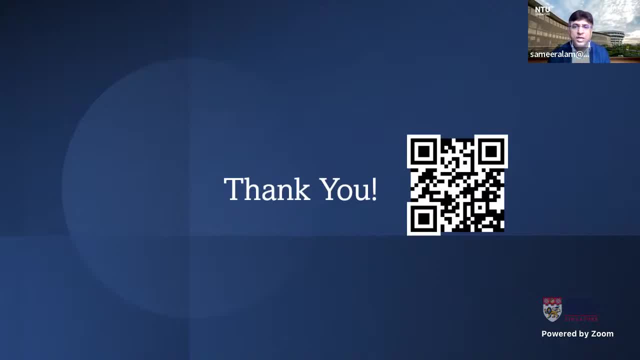 skills. you are ready for it. Most of the FIP projects that are done now in the School of Mechanical Aerospace Engineering touches on the soft side of aviation, making use of data science, See. data science is a ubiquitous reality of our daily life now We cannot ignore it. 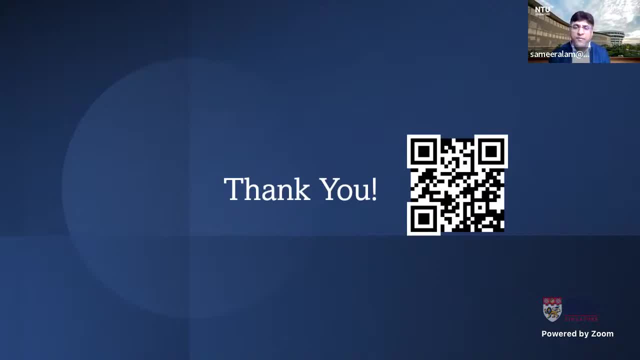 We in the School of Mechanical Aerospace Engineering have embraced data science Four years ago. our students who are graduating now are finding not only jobs in the aerospace industry. they are data scientists in Shopee, data scientists in Seagate, data scientists in CASS. 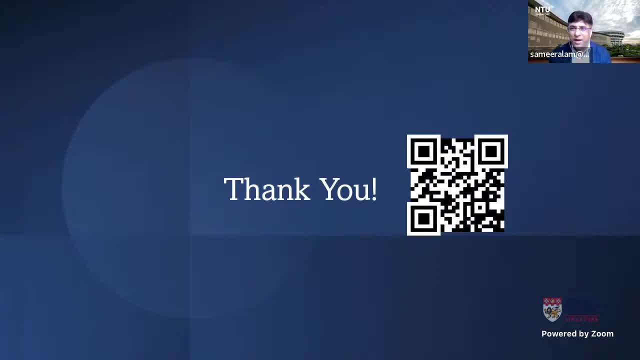 data scientists in the Changi Airport Group And how they achieve that. Because they have this cross-domain knowledge, Both of data sciences as well as of aviation air traffic management, And they were the ones who are acing the interview- They are better placed. 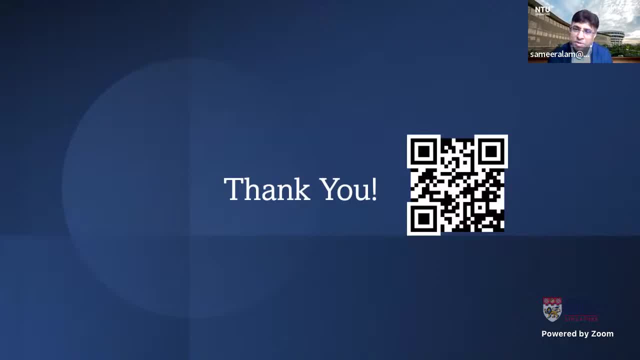 than those who are just trained in programming or computer science background, because they come with the domain knowledge And they are also better trained from the students who are just trained in the aerospace hard aerospace engineering from other universities. In MAE you have the advantage of: 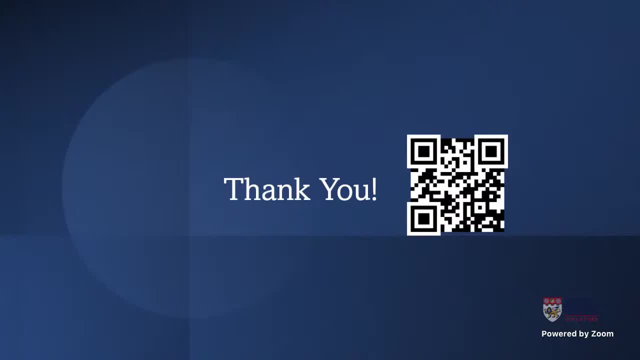 this dual training, Both on the soft side and the hard side of the aviation. So I'm sure when you will graduate from MAE you will be very well equipped. We will make sure that you are equipped to tackle any challenge, any demand of the jobs when it 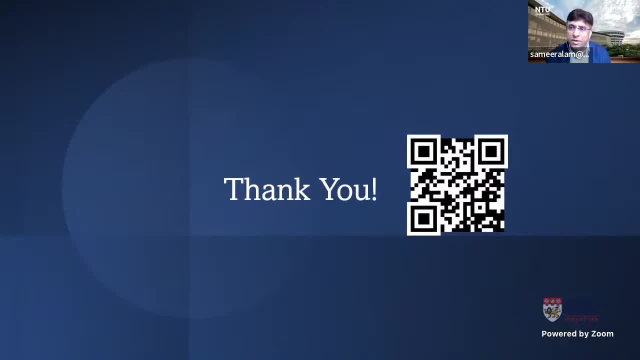 comes to the future industry 4.0. Thank you. Thank you, Prof Samir. So this is all the time we have for today. If you have any other questions, feel free to keep them coming on. Slido- Slido will be live today from 10am. 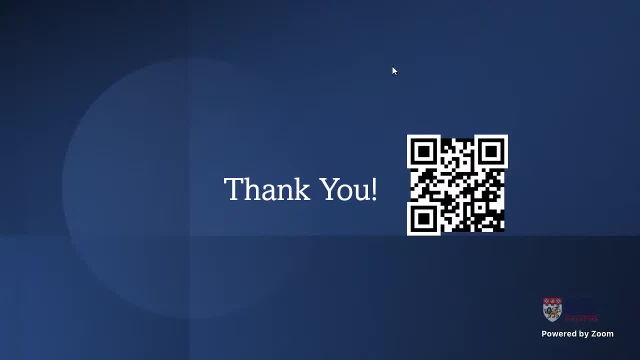 to 5pm And we have a group of students and staff and professors online to address your questions. If you have any questions directly just for Prof Samir, feel free to let us know as well in our email address And we can redirect. 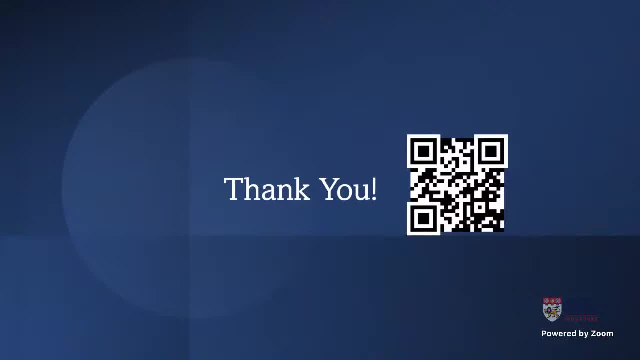 them to Prof Samir, if required. So, everyone, thank you once again for joining us today. I hope you have had a fruitful session And I hope to see you in NTU soon, Thank you. Thank you, Elaine. Thank you, Edmund, It was such a nice.